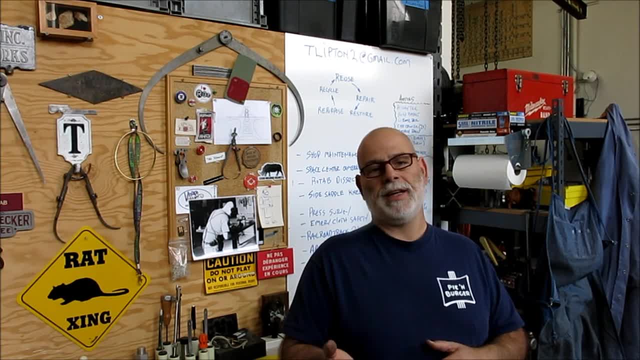 showing. here is a technique for joining stainless steel to brass or stainless steel to copper, Which can be a tricky joint. This material melts at a lower temperature and and behaves much like soldering or brazing, but with TIG welding, so without the messy fluxes and whatnot. So I got. 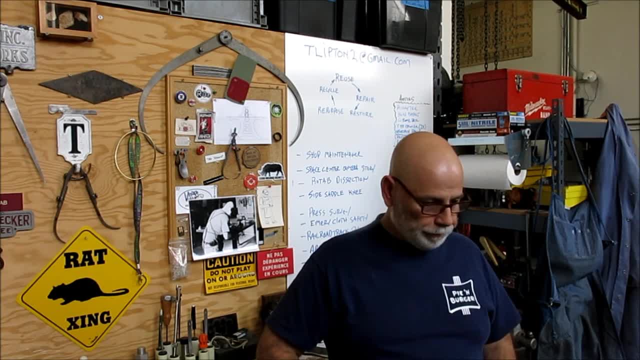 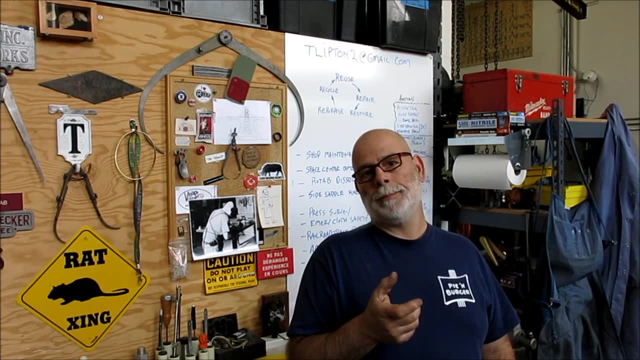 some bits cut over here at the welding table and we'll do some test joints and then a couple of things: The joint that we did with the silicon bronze, which is the first part of this series, and we're going to take a look at that too. We'll bust that open and get a look at the weld there. 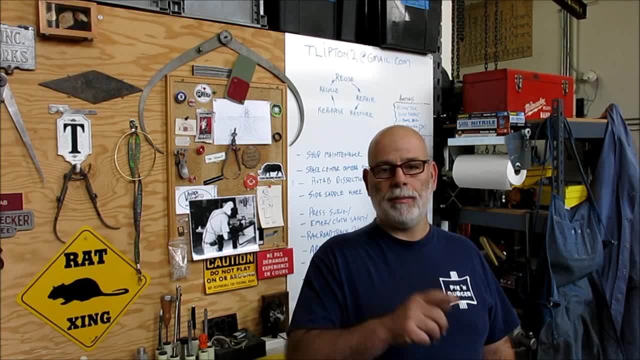 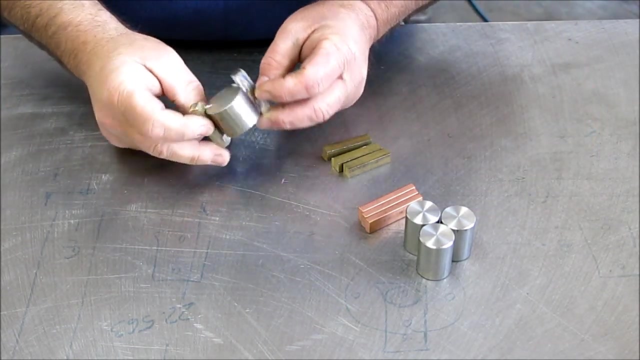 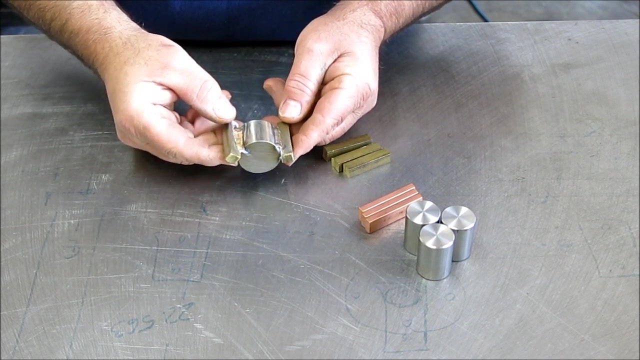 So I'm practicing my arc welding on video, so we'll see if I'm improving there. So I'm trying. Anyway, let's get an apron on, Let's go over to the welding area and let's put some stuff together. Okay, so here's the sample that we did in the first video: Welding dissimilar metals with TIG. 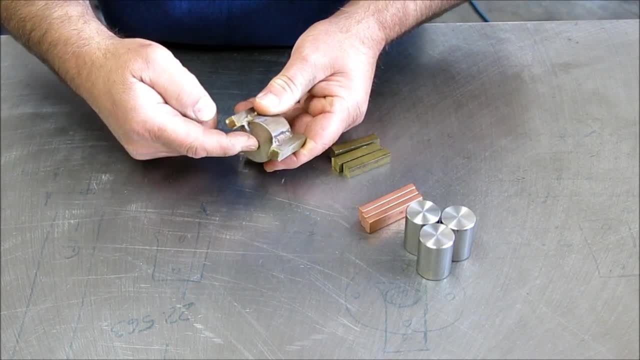 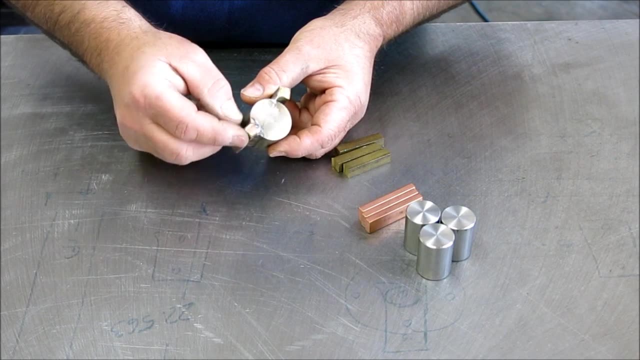 welding, And so we have 360 brass to stainless steel And we got some welds on there, and a couple of viewers suggested that I try to break these, which we're going to do. I think that's a good idea. We'll see what this looks like. 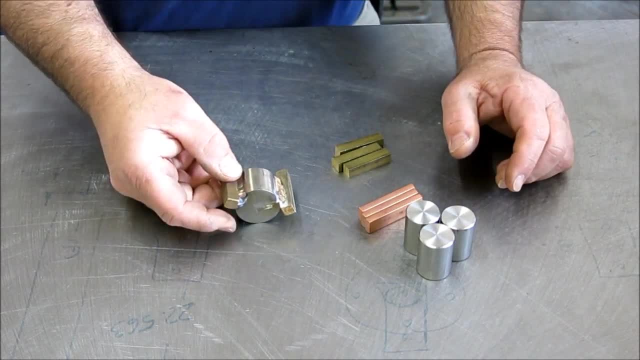 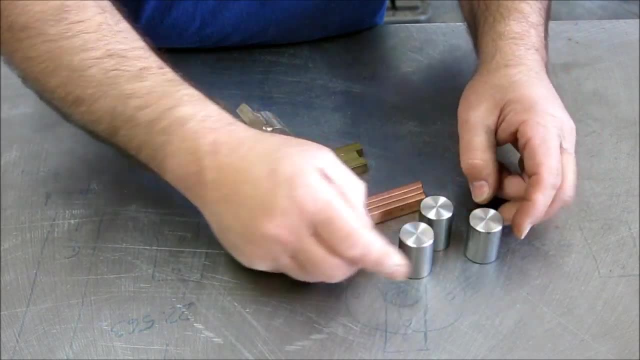 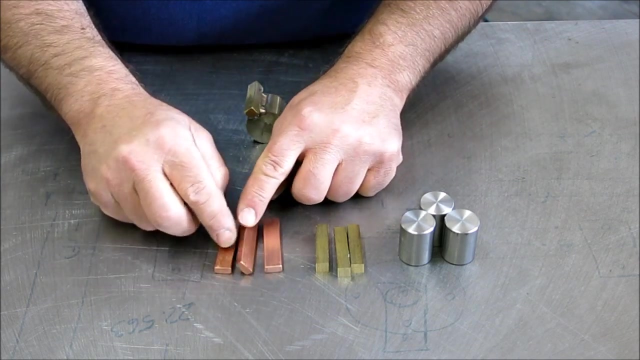 But I also wanted to show a different kind of rod also. We'll get to that in just a second. So I got some more blanks set up here. These are stainless steel, That's 360 brass the square, And then this rectangular stuff. this is copper here. So we're going to do a couple different joints here. 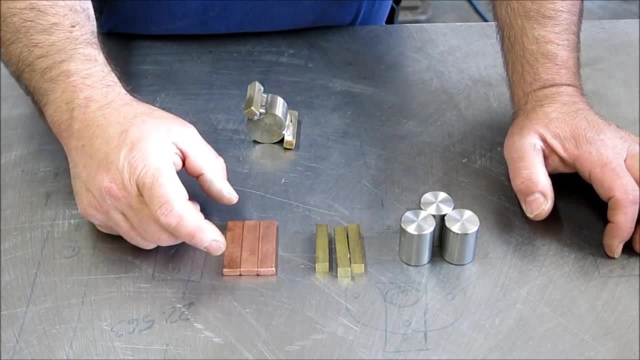 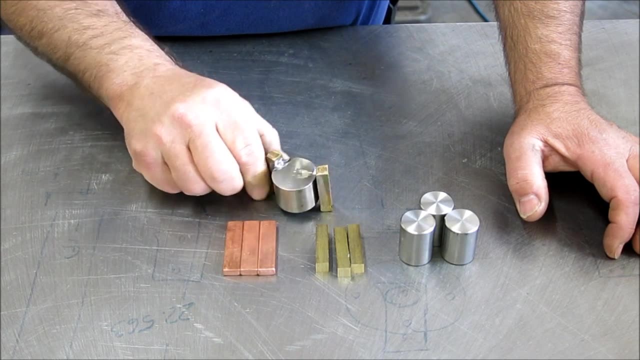 with this other material that I'll talk about in just a minute, But meanwhile let's take this over to the vise and see if we can break that and get a look and see what that weld looks like. Okay, so we got this in the vise here. 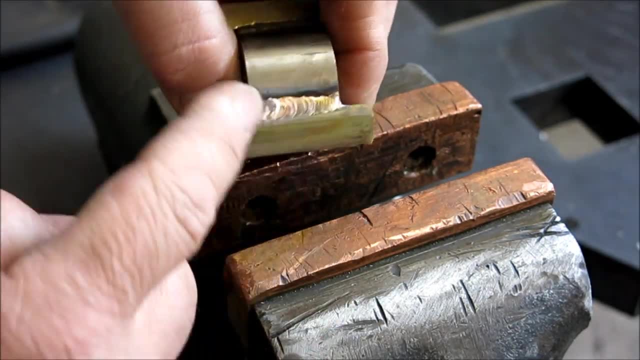 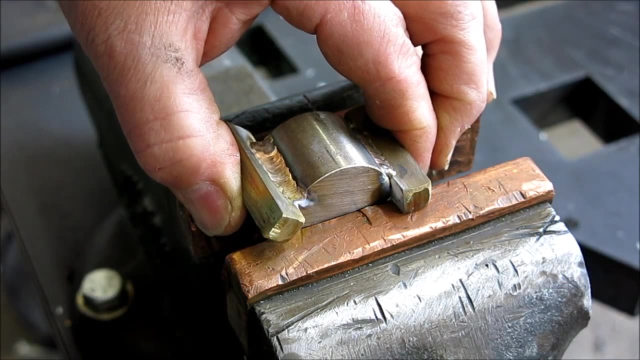 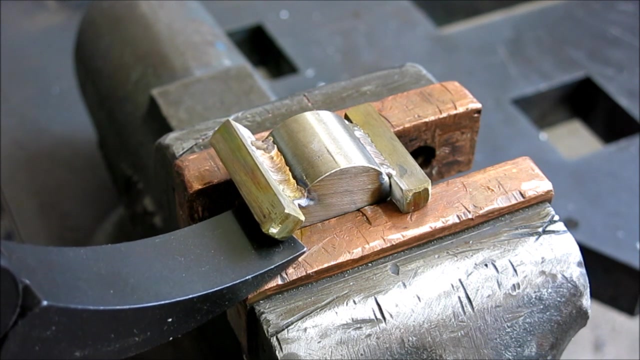 This one's welded on both sides here, So I'm going to pop this one loose, since it's welded on one side and will probably be a lot easier to pop loose. Let's set that in there, Get that in there, pretty good, And I'm just going to use a pry bar here. We're just going to try to lever that off. 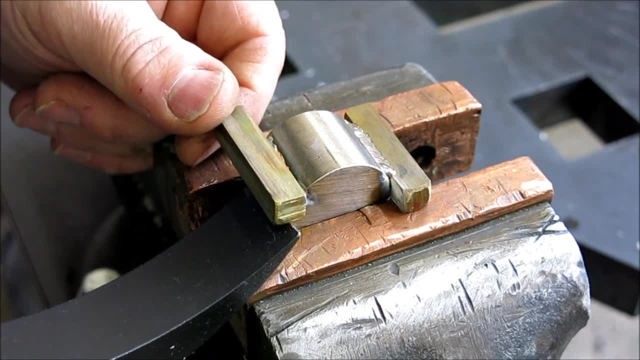 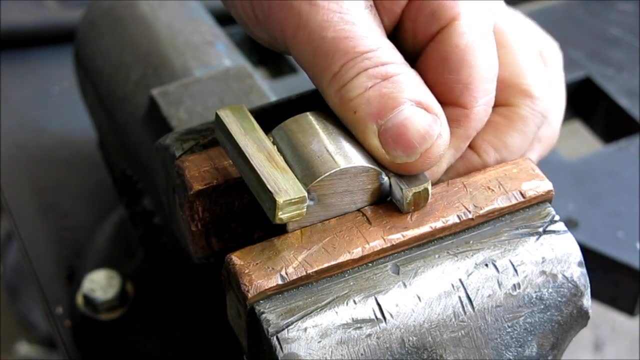 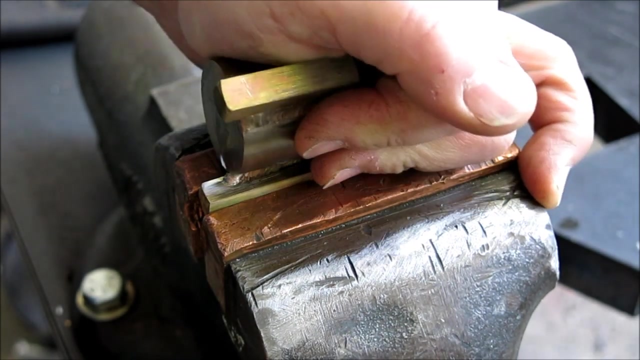 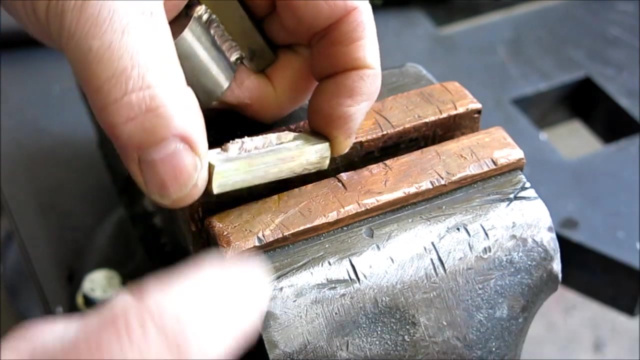 see if it's coming right off. Okay, so it's loose enough that I can All right. All right, so it's failing on that side. See if we can get that up there. Well, it's failed kind of right through the. 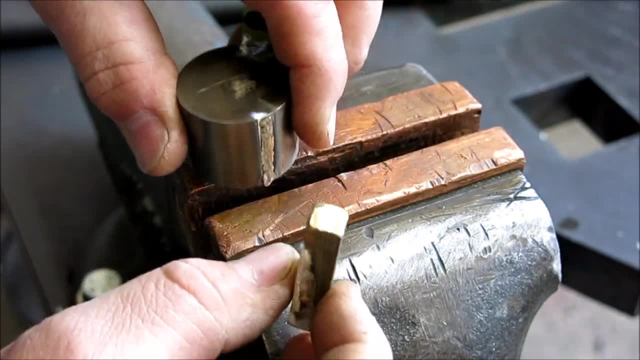 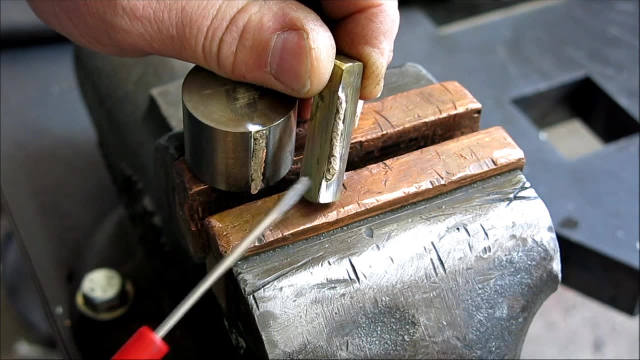 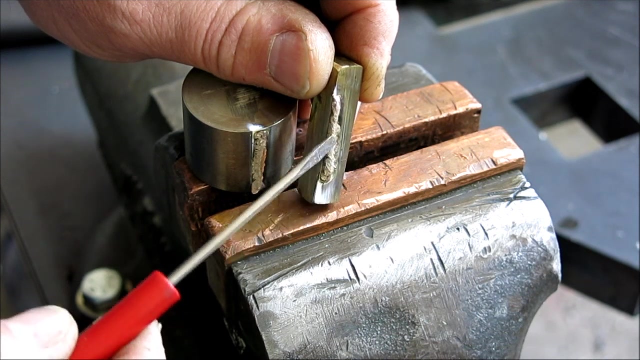 the silicon bronze material, which is actually kind of good. So its connection to the, to the base material, seems to be pretty good. So we've, you know, these materials dilute. well, the lower temperature materials dilute themselves a little bit. So that's actually. 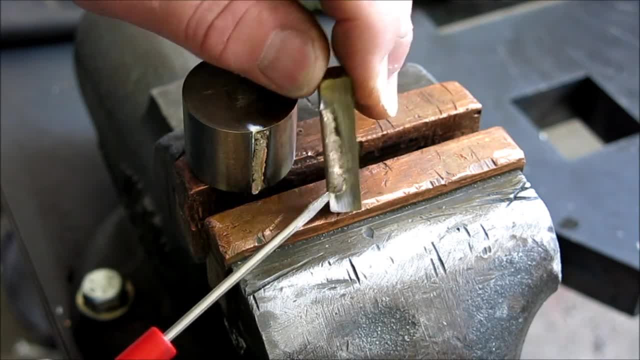 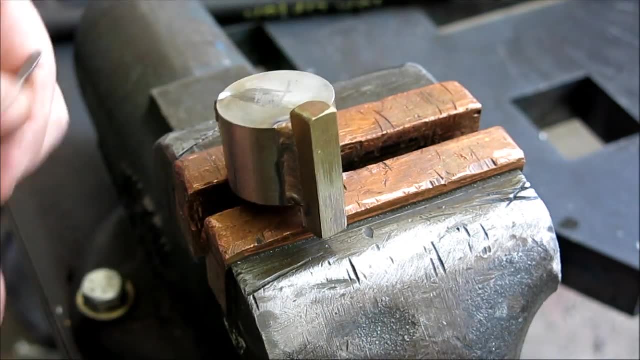 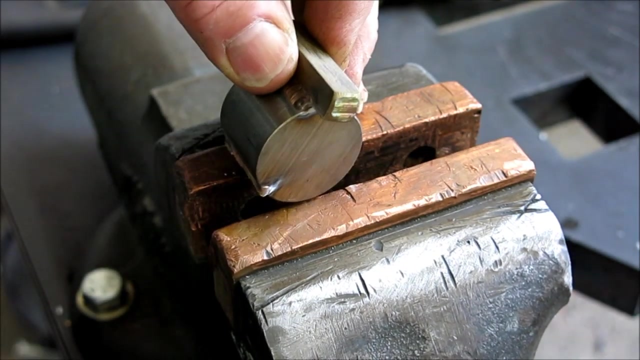 not bad, That's. I kind of expected it to pull out of the brass myself, but that was pretty good. Let's, let's, let's try doing something to that one and see if we can get that one. Now, this one's welded on both sides, so that's probably going to take a little more. 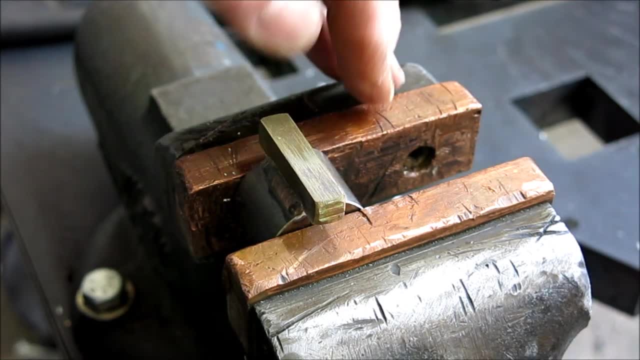 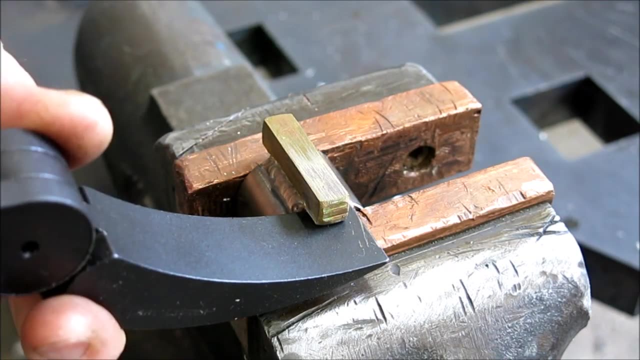 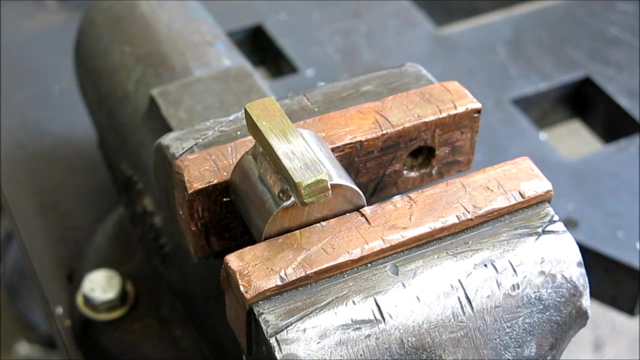 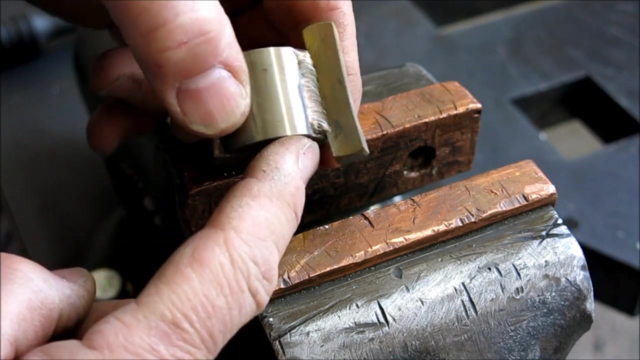 a little more elbow grease there. Let's try this. I got a pretty good purchase on that. I'm getting my snap-on pry bar in there. I think I'm just pulling it out of the vise now Bend that. So that's quite a bit of force to actually bend a 3-8 brass thing that close. 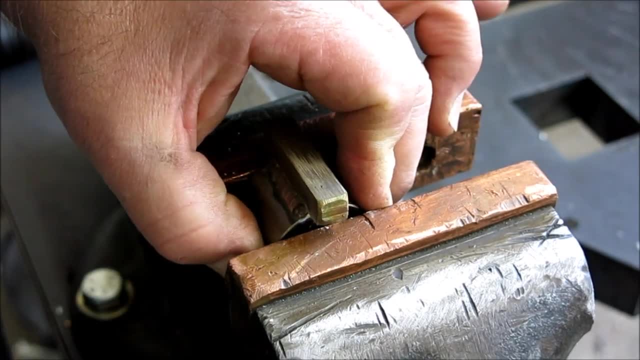 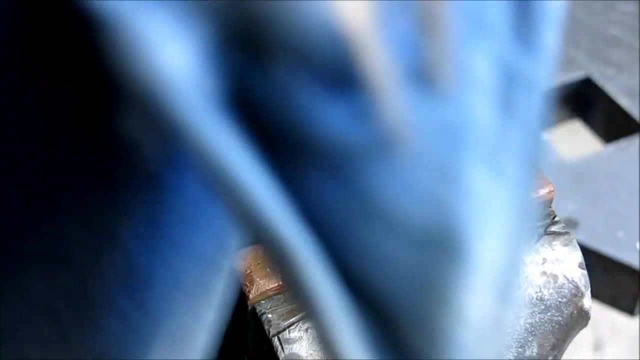 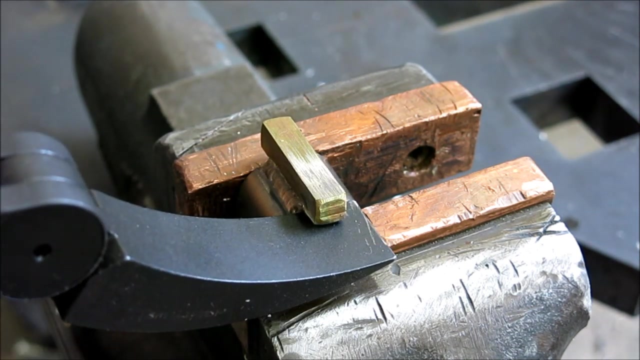 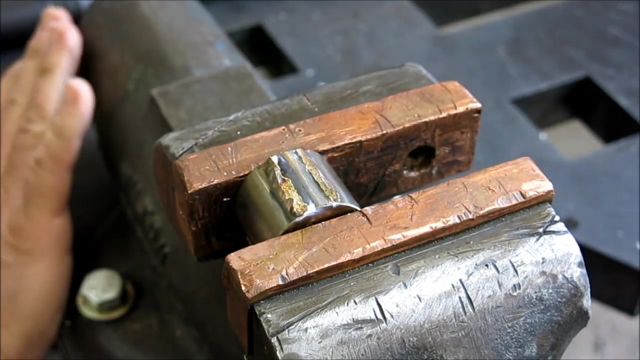 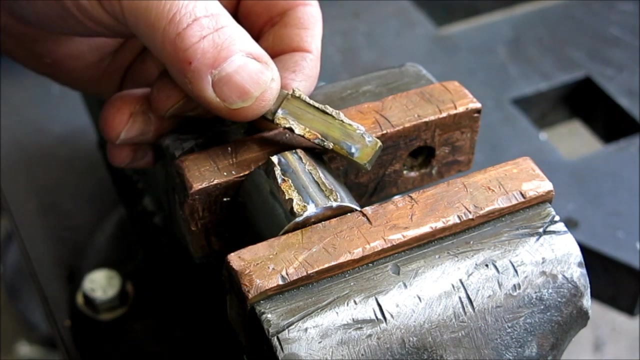 Let me, let me try that again. Let's see if I can get at the break. I got to put some, put some gronk on that. Let's try that again. Okay, so I did it a little more suddenly and once again it broke on the filler interface there. 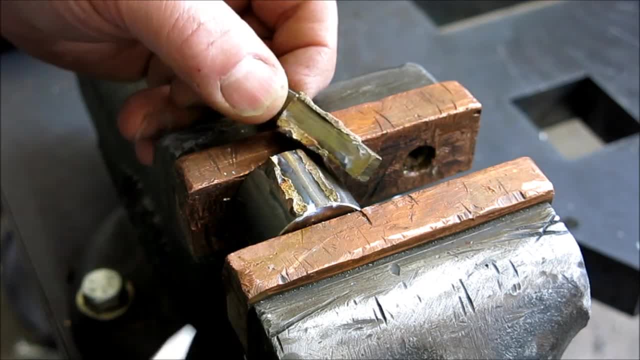 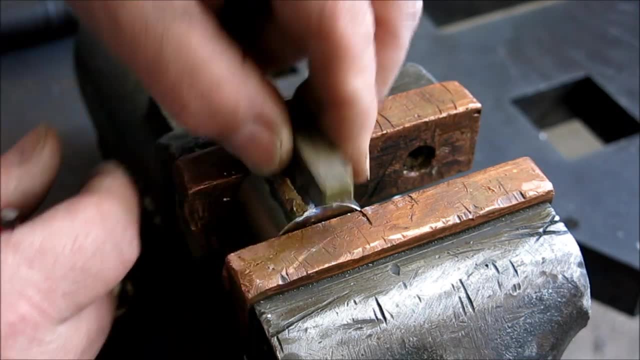 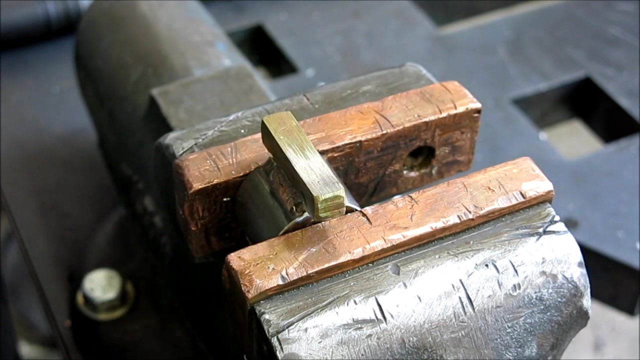 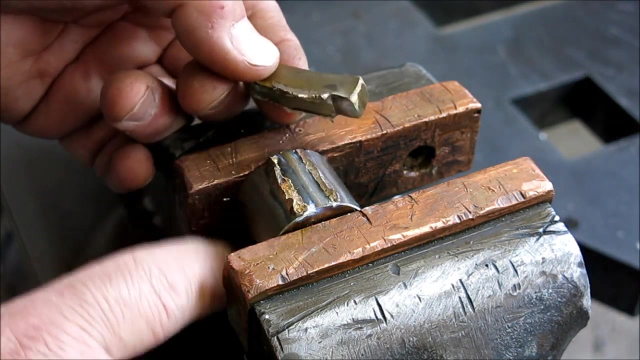 which is kind of good. Can you see that? it's a pretty good shot? So that was actually a fair amount of force to get that to break. I wasn't being shy on that and it broke right through the filler material. Anyway, I'd say that's a pretty good joint, considering brass is a pretty wimpy material. 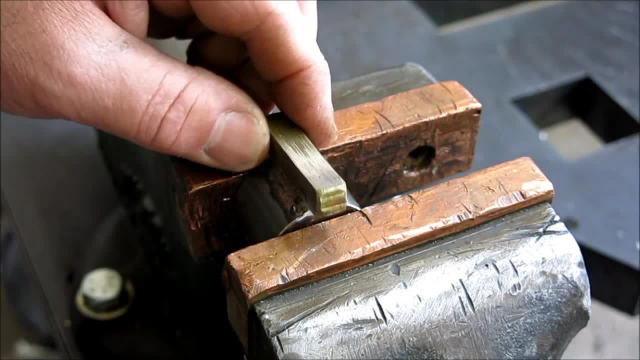 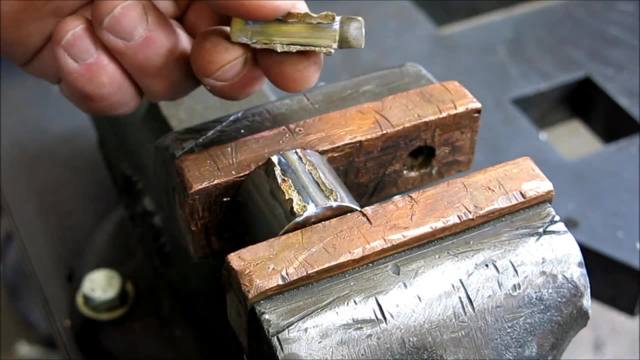 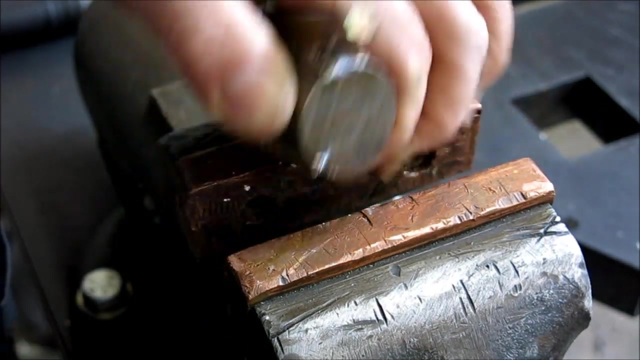 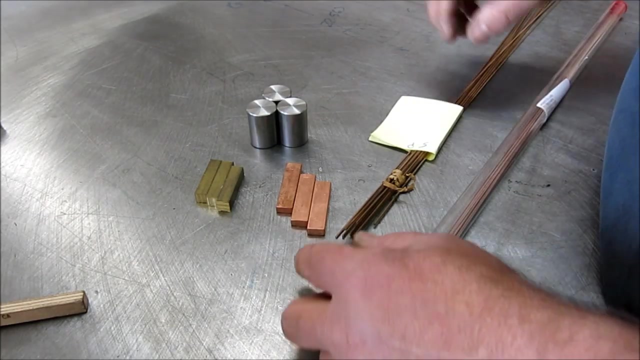 stainless is certainly stronger, So you're not building a crane with this technique. This is more of a decorative type welding application. So got some strength. how much kind of hard to say Okay. So here's our samples again: stainless steel, 360, brass and copper. 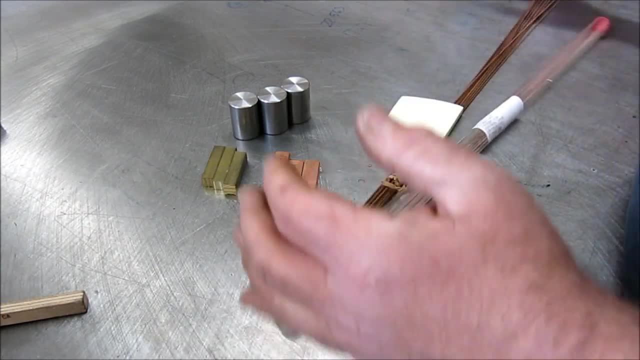 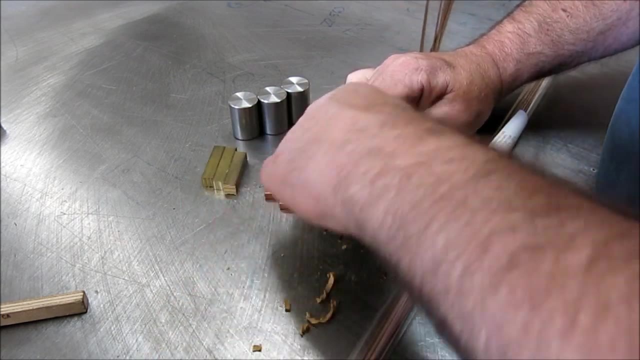 And this is the rod that we're going to use here, And what this is is. this is basically a silver brazing alloy and it's got a really bad rubber band on it. All right, so we're not going to use that end. 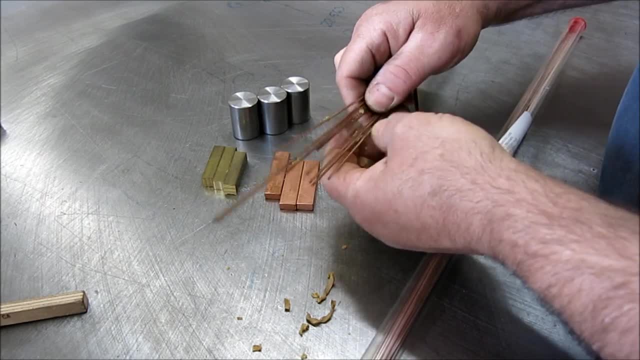 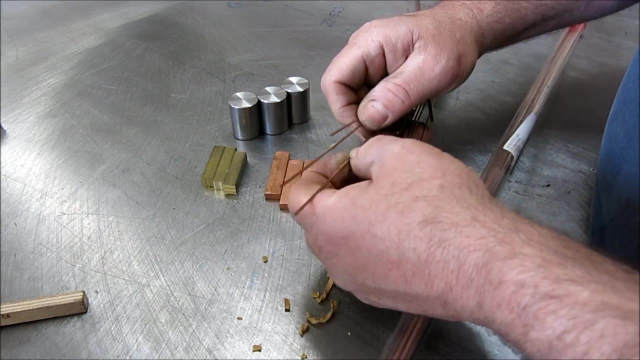 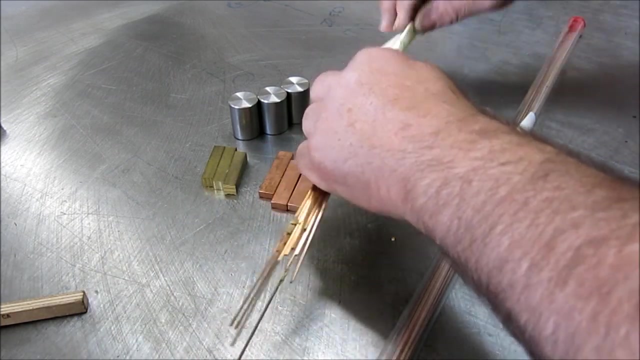 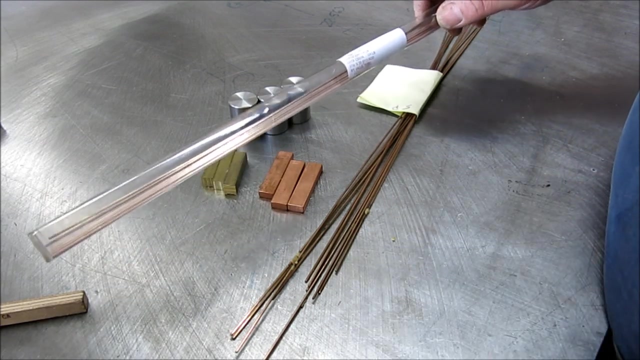 So there's a reason to not use a rubber band to hold the rods together. Kind of left a residue on there that's probably not conducive to welding. so all right anyway. So this particular rod here. there's two alloys here. This particular one is 15% silver and then the rest is copper and then a little bit. 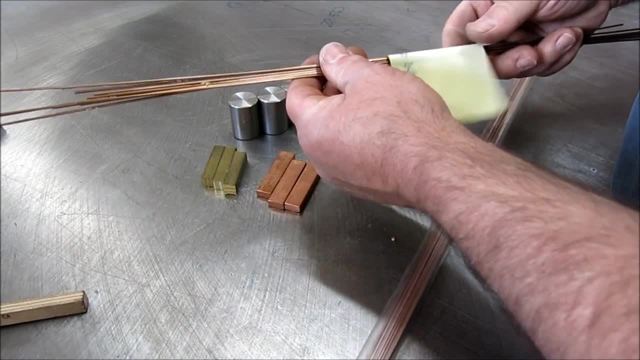 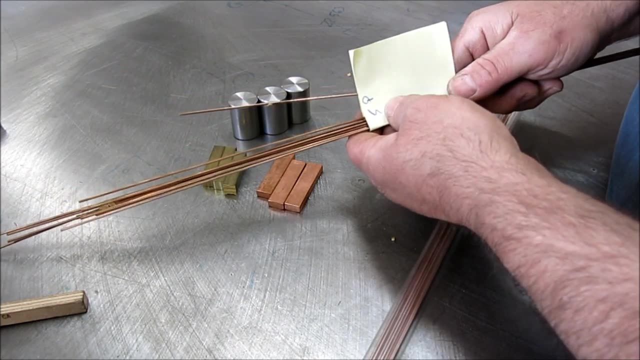 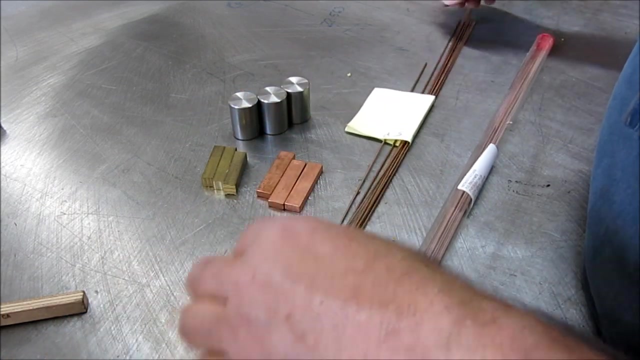 of phosphorus. This one has a lower silver content, So it's 5% silver, 89% copper And 5% phosphorus. So these are silver brazing alloys that you would normally use with a torch and on flux and that kind of thing. 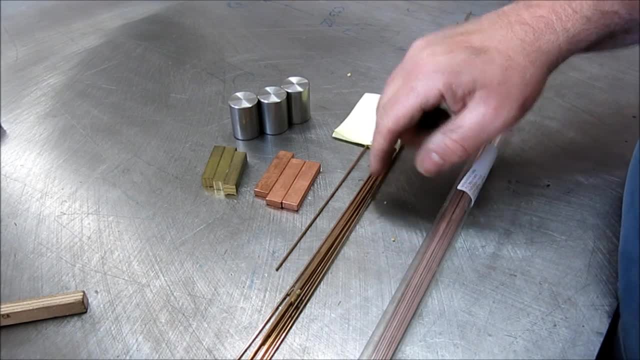 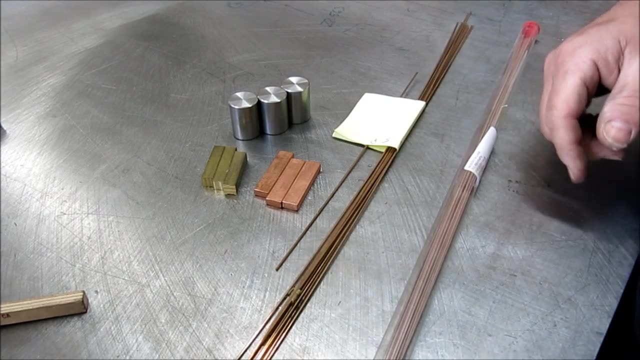 But they actually work really well for joining dissimilar metals at low temperatures with TIG welding. So I want to show these and we're going to duplicate that joint that we just broke a little while ago. We'll kind of do the same thing. 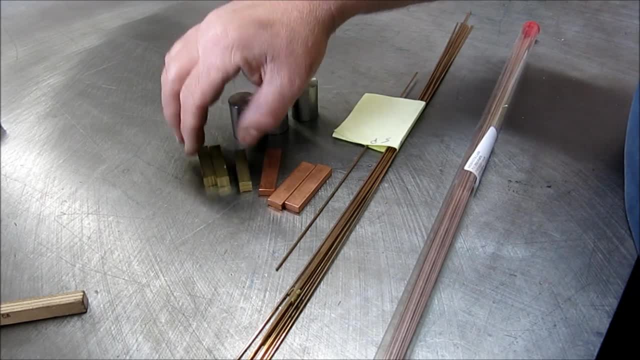 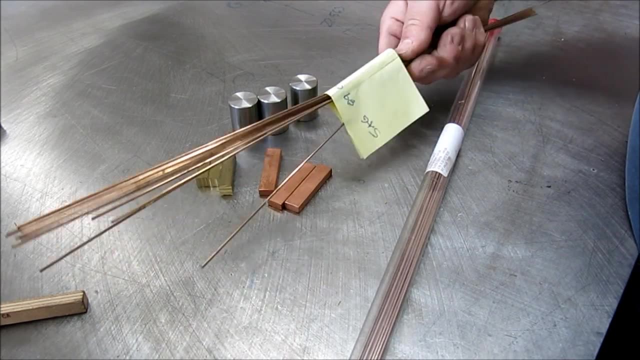 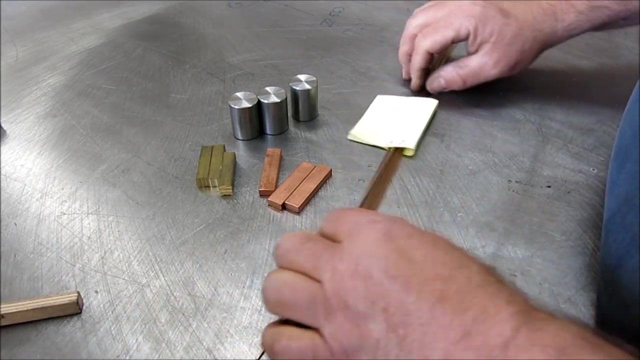 We'll probably do one copper And one brass. I don't know if I'll use both rods. I'll probably use the cheaper. This is cheaper because it's got less silver in it. We'll use this one And I'll put the part numbers at the end of the video so you guys can see it. 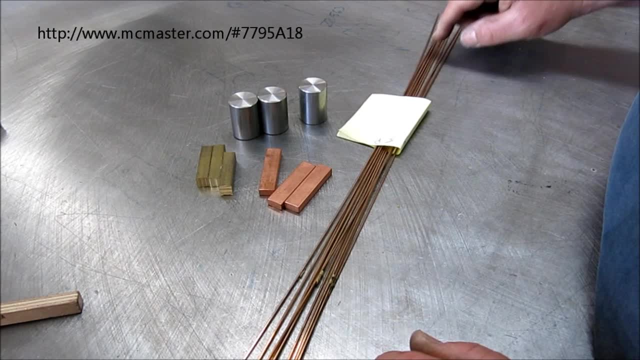 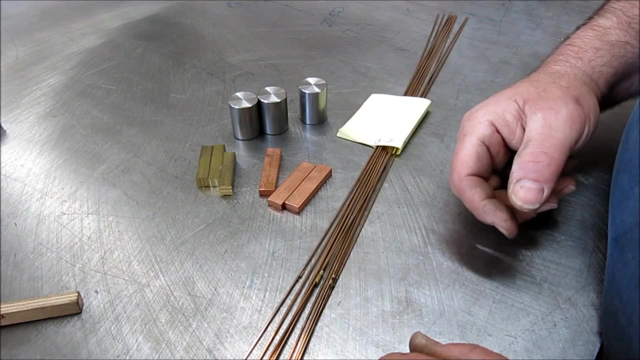 And I'll try to get some arc shots here so you can kind of see how this stuff behaves. And then we'll try busting these joints and you guys can get a sense of how this stuff behaves. And I've got a little bit of silicon bronze left, which is actually another good rod to. 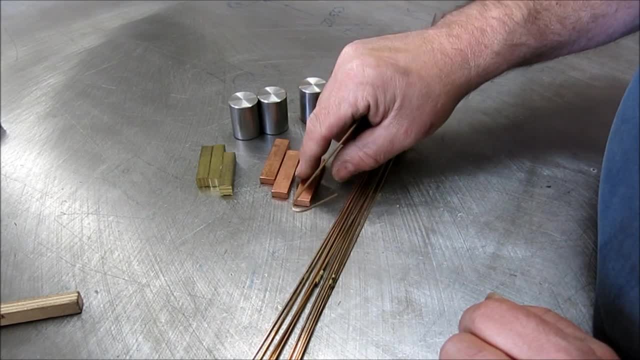 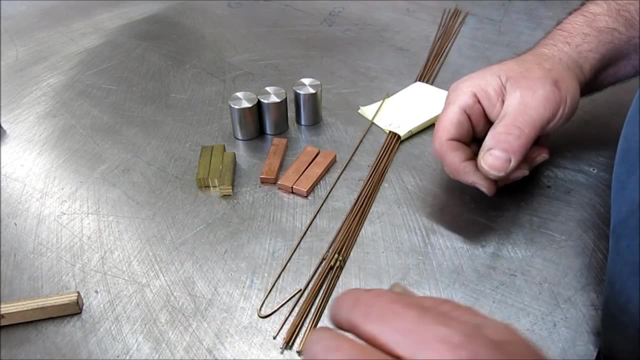 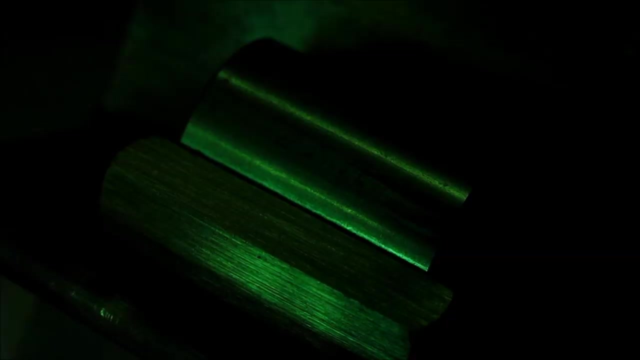 join copper to copper. Maybe I'll find another piece of copper and we'll do a straight copper to copper joint with silicon bronze too. So let me get set up for welding here and then we'll do some welds. All right, so we're going to try this. 5% silver brazing alloy, 360 brass to stainless steel. 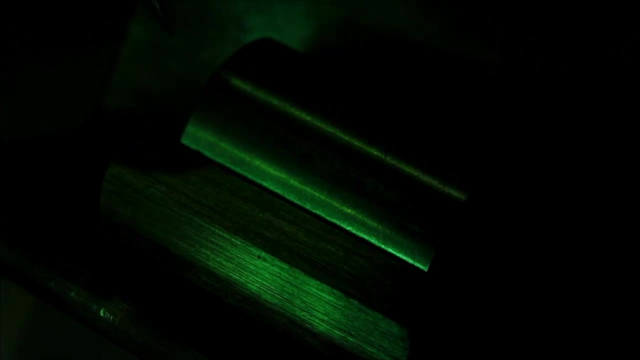 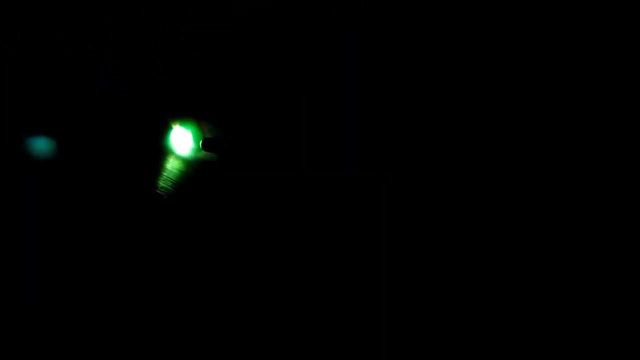 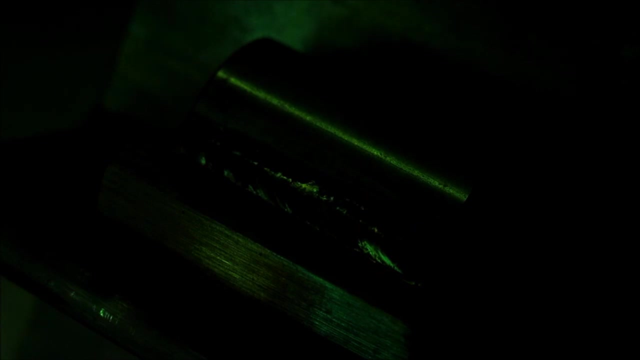 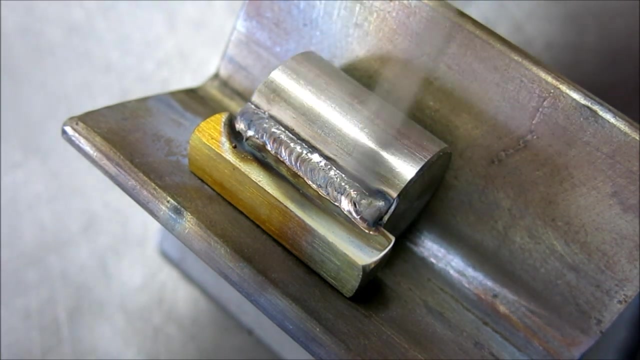 All right, Let's go. Okay, so you can see that came out pretty good. So this is the 5% silver, 89% copper, 5% phosphorus. So we didn't get. we got a little bit of zinc fuming here. 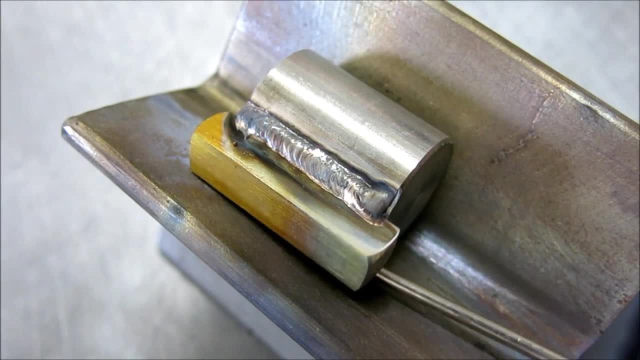 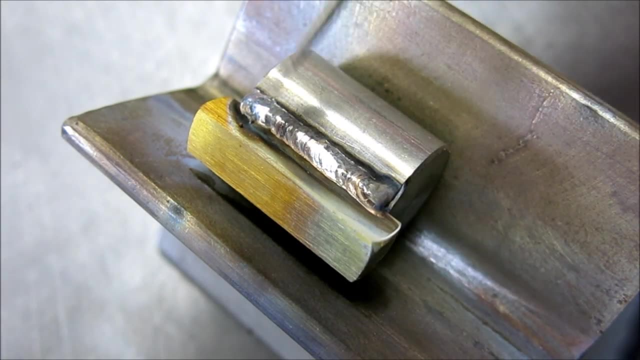 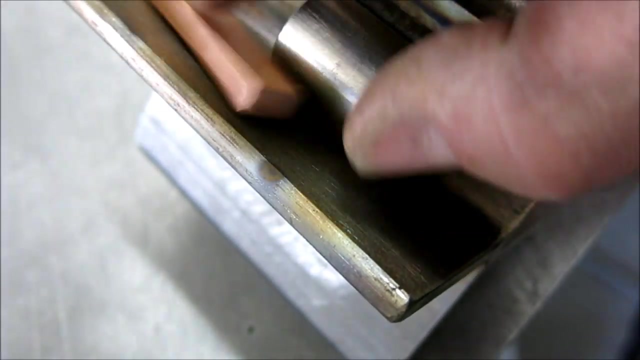 So you can see that this is already a lower temperature type joint and that stuff lays in there pretty good. So what we're going to do now is I'm going to leave that one alone, I'm just going to turn this around and on this same piece we're going to go ahead and attach a piece of copper. 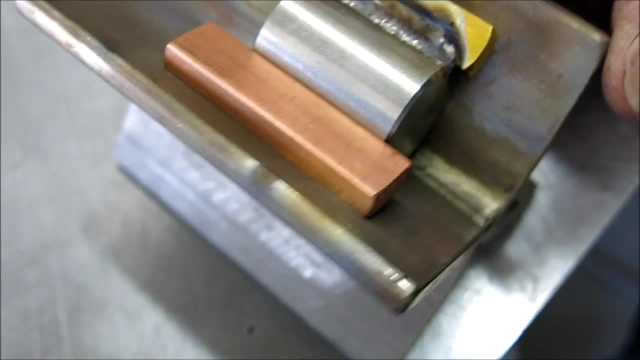 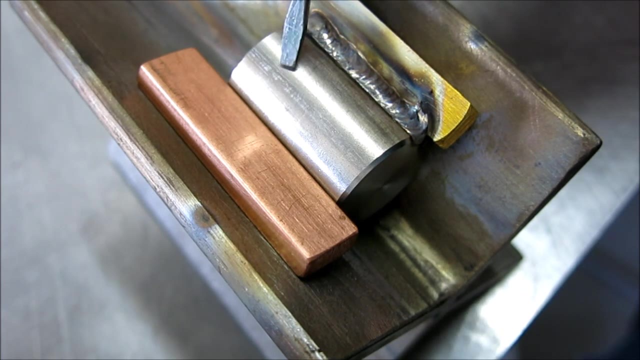 here as well, to kind of continue on with the test here. So we're going to weld copper to stainless here with this same piece, Some rod, And then I think the final will be the copper to copper with the same material, the same filler material. 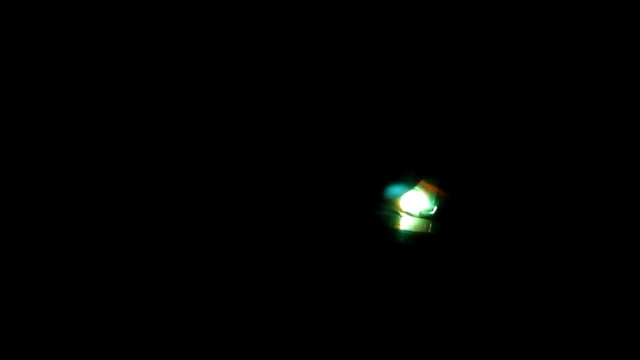 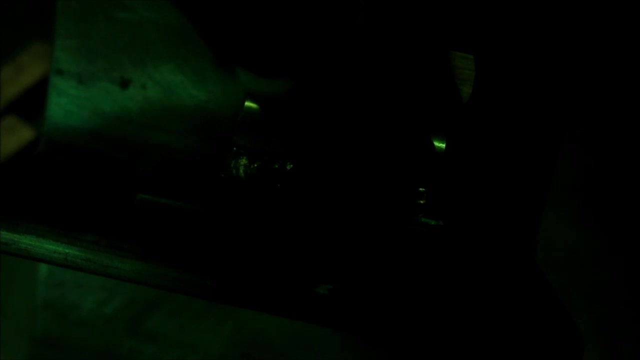 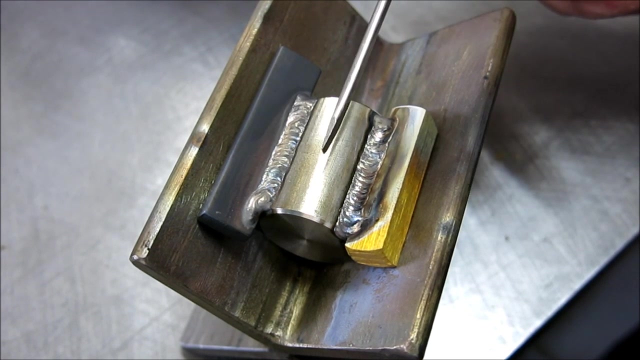 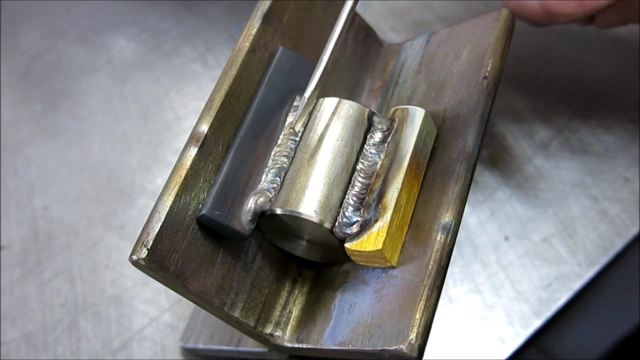 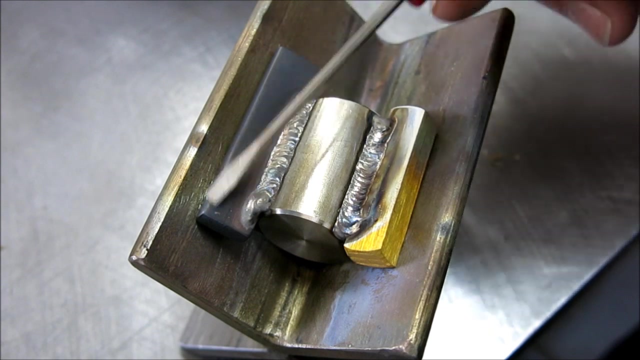 So we're going to do that, Okay. so here's stainless steel to 360 brass and then stainless steel to copper And this is with this, 5% silver, 89% copper, 5% phosphorus rod. Now this piece got pretty hot just because it's copper and it conducts heat real well. 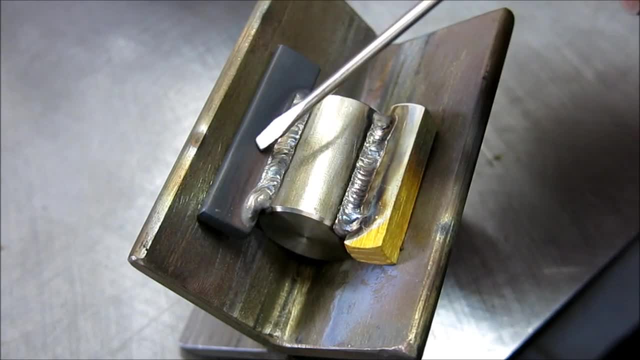 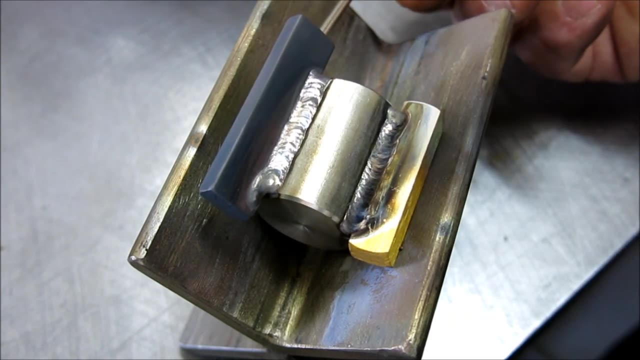 But it's basically a low temperature process. This need not get to melting temperature to do this process. Anyway, I'm going to let this cool off a little bit. I'm not going to weld the backside here, because what we want to do is we want to try to break. 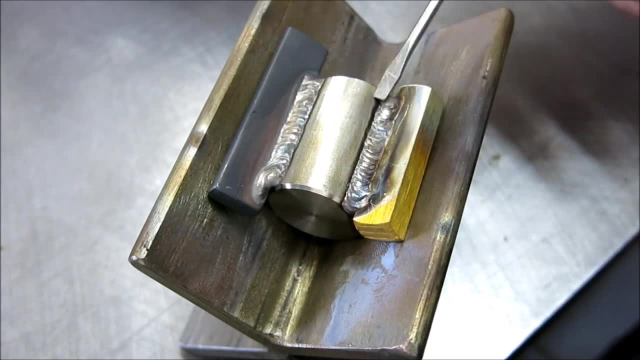 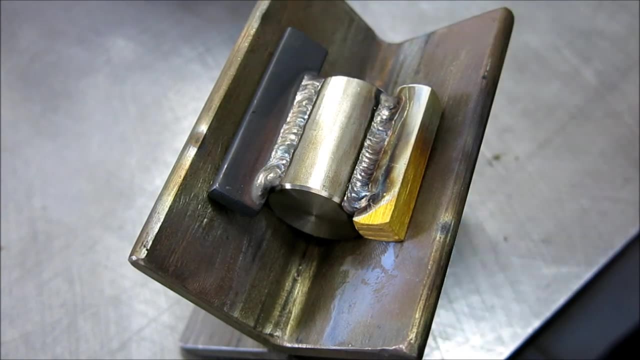 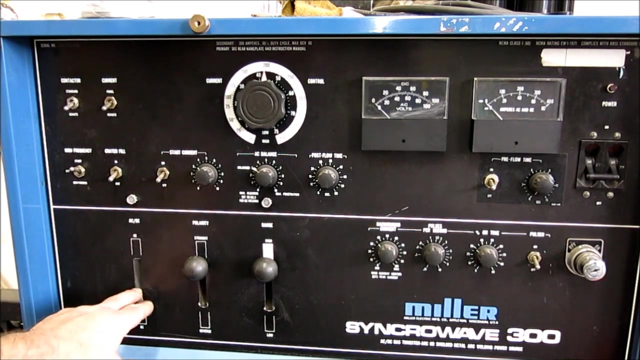 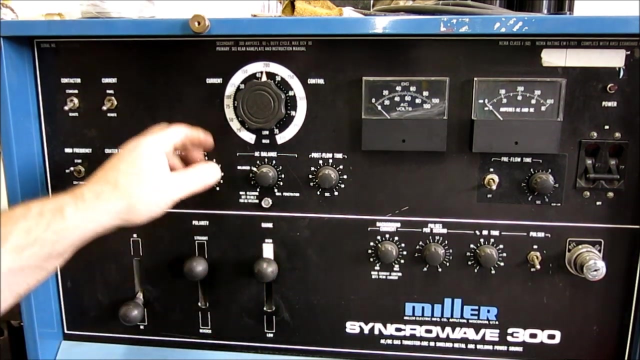 these off and see what happens when we break those off. Okay, So the last joint that I'm going to do is copper to copper with the same material here And we'll see how it behaves. Okay, Okay. So here's the basic machine settings: DC polarity. we're straight, I'm in high range. 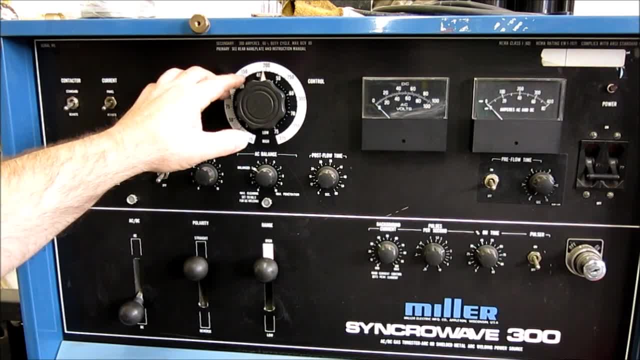 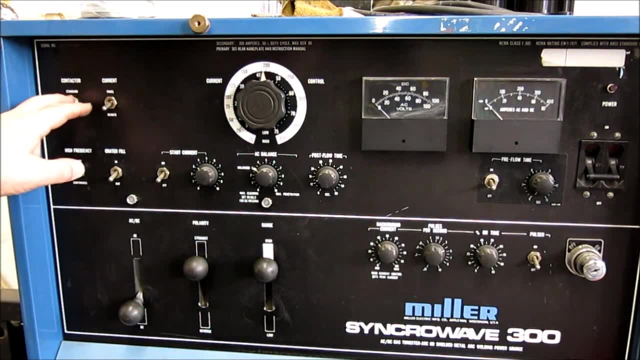 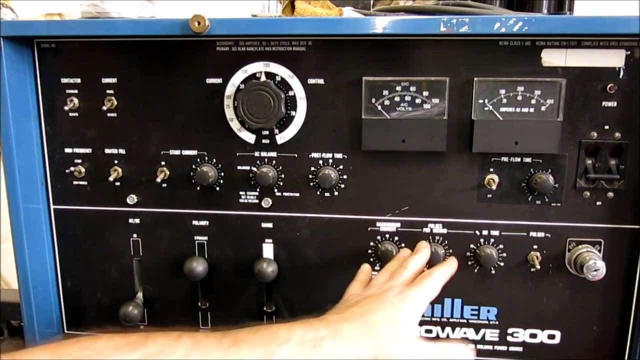 and I have my main current control set kind of at a maximum, of say, 200 amps, although I'm controlling it with the foot pedal. Okay, So remote current control, which is foot pedal, just a high frequency start, no, pulsing, no. 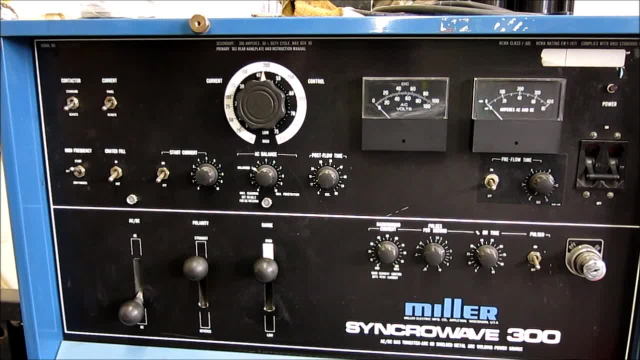 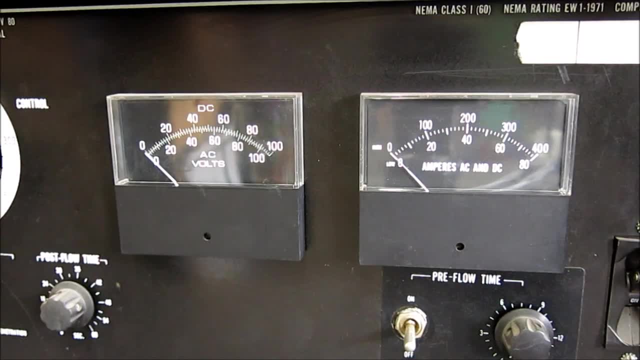 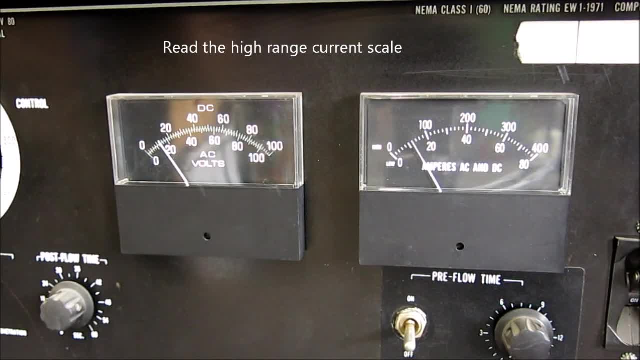 You got two minutes to help me resolve the problem. Okay, All right, All right, Okay. What am I going to do next? Okay, Great, Alright, Okay. So let's start vedere and talk a little bit about IntelHz. 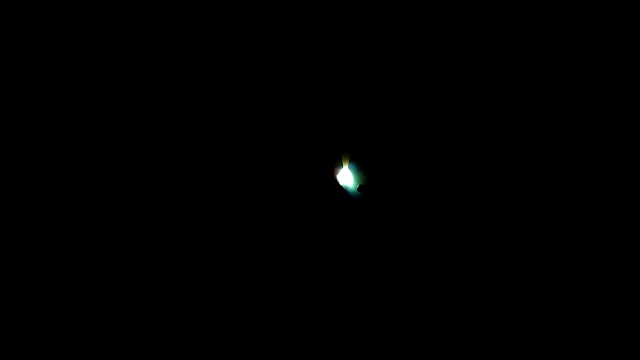 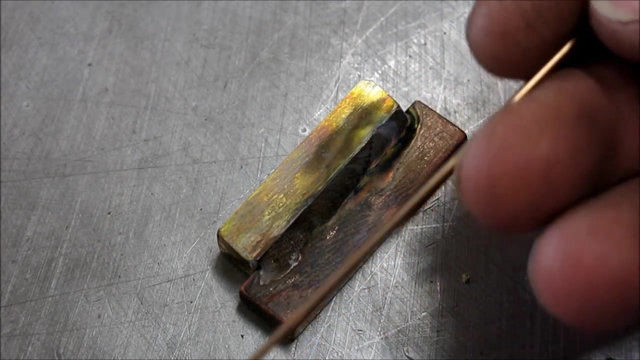 governments and about IntelHz. Okay, Okay, Awesome, That doesn't. he got everything? Nobody, Okay. so this is the 360 brass to copper with this silver brazing alloy. Now, I haven't done anything other than just cool it off. 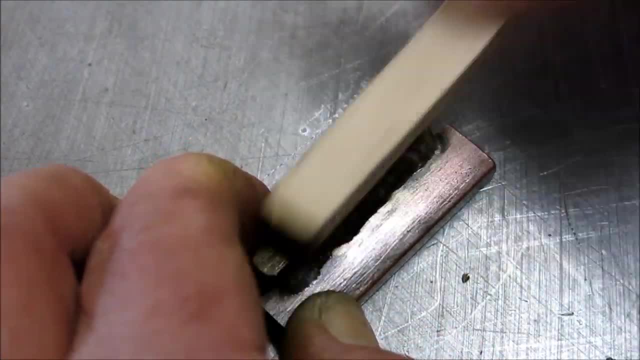 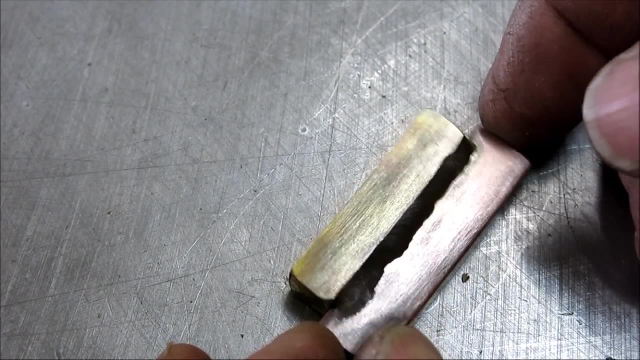 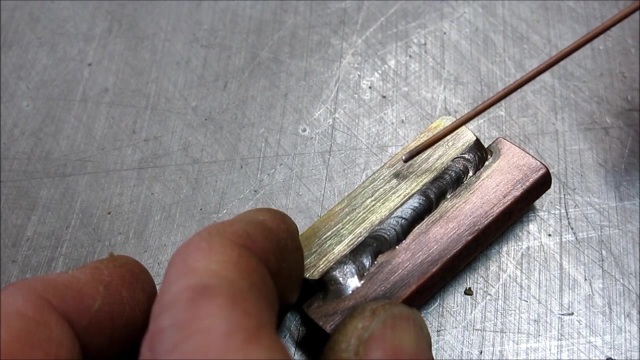 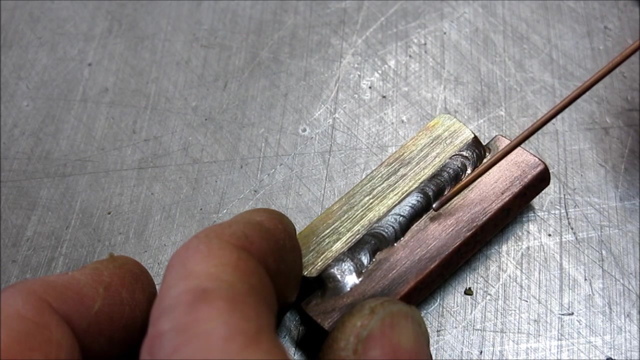 Now I'll brush it a little bit Now. one issue with this particular rod is it doesn't have a good color match between copper to copper or brass to brass or copper to brass. It ends up with kind of a dark. the weld is darker colored, so you don't get a good color. 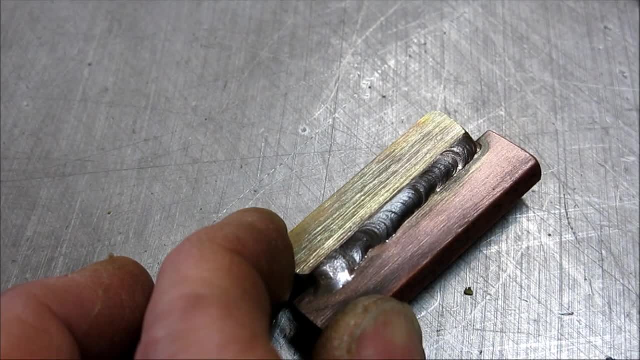 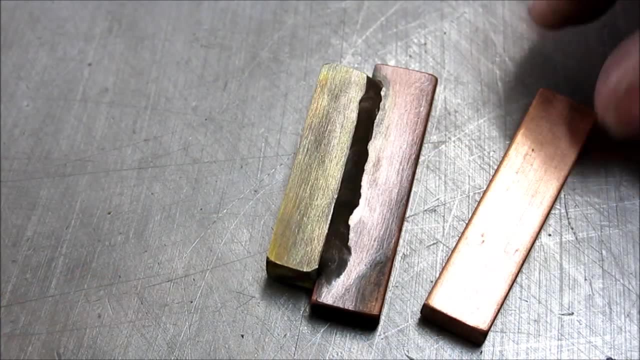 match. That's something where that matters. okay, and sometimes it does matter, Okay. so we did this 360 brass to copper, and then the last one we're going to do is we're just going to do copper to copper here, like that, and I'll leave it open a little. 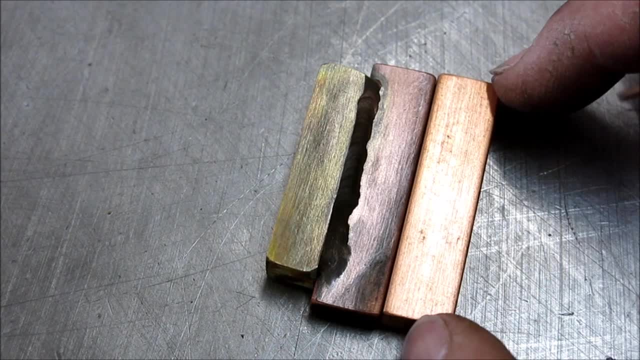 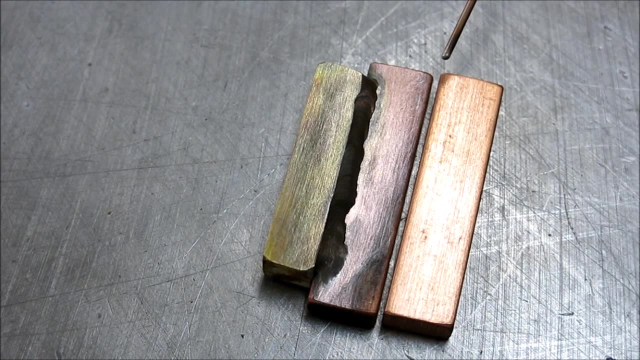 bit like that. It just makes the weld go a little easier instead of trying to generate enough heat to get it to flow there. So we'll leave a little gap like that and we'll just run a little weld along that and see how it goes. 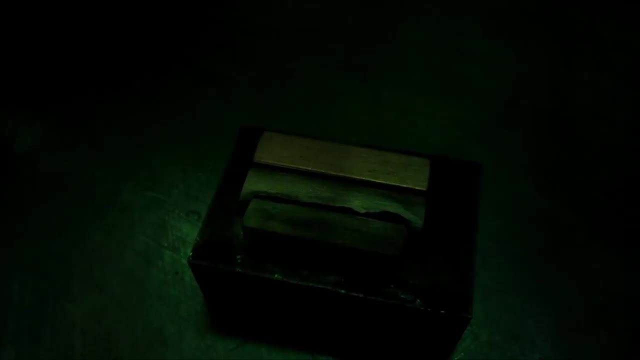 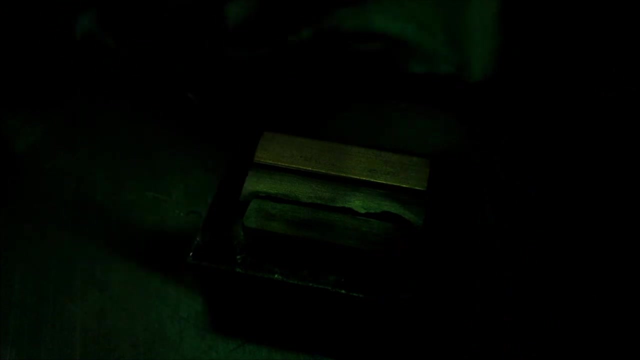 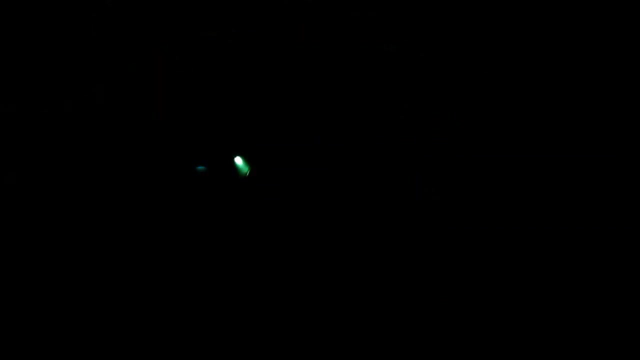 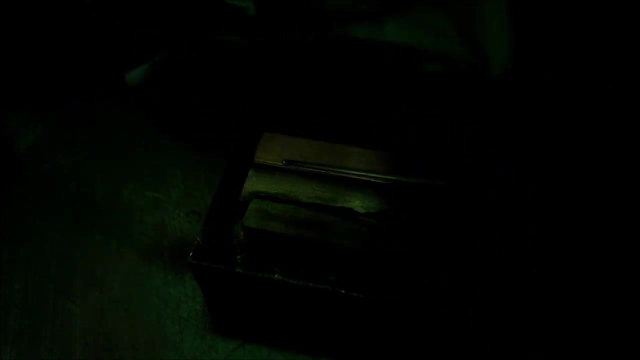 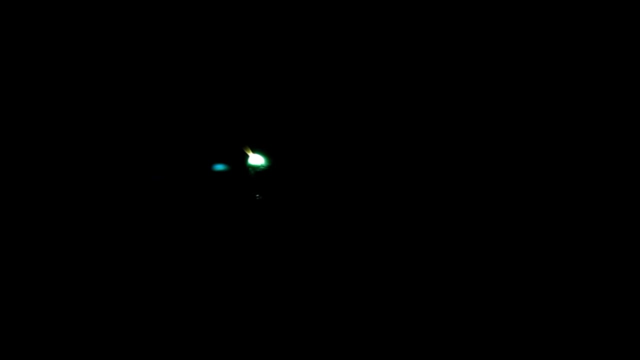 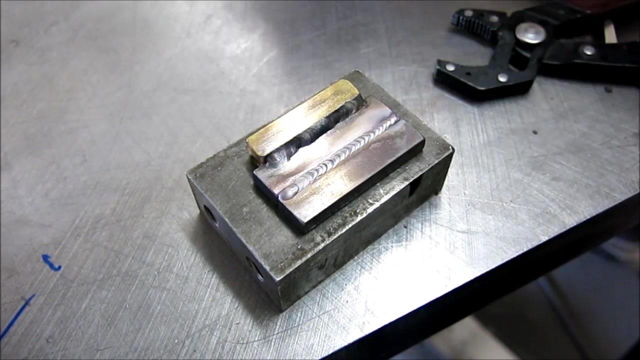 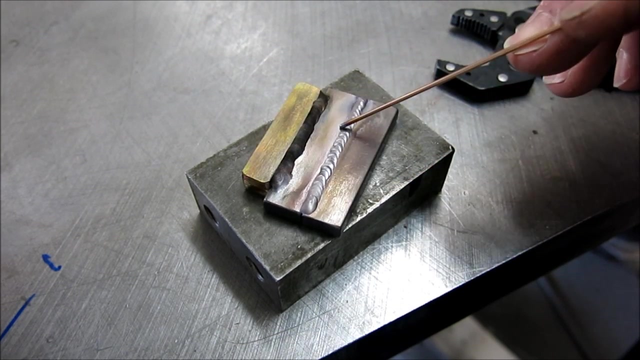 I don't know, Let's go. Okay. so this thing's still hot here. This is the copper-to-copper that we just did, and I'm going to go cool that off and then we'll brush it. I'm going to hit it on the power brush. 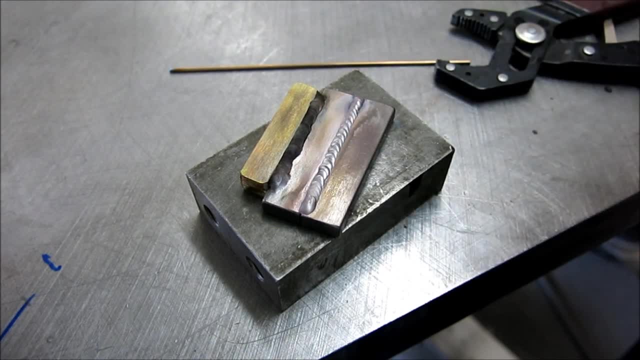 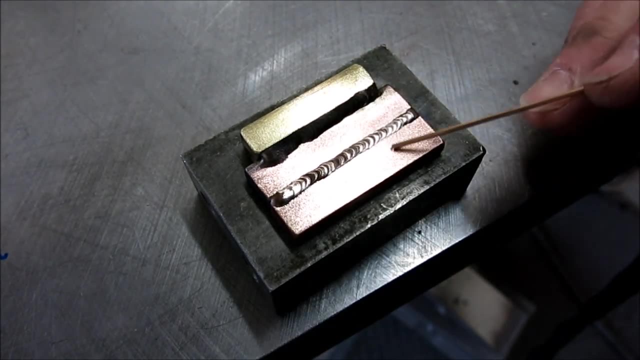 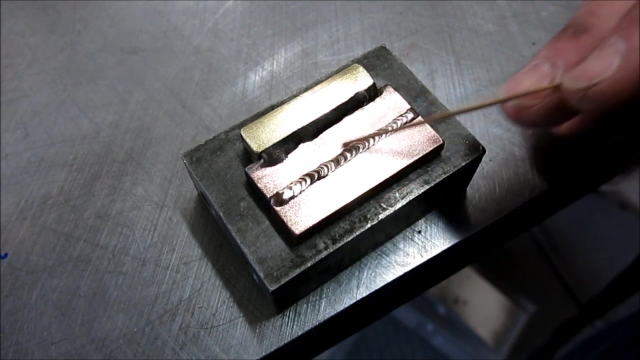 That way you guys can kind of see this color match thing that I had mentioned earlier. So let me cool that off and I'll brush it. Okay, so there it is polished up. It's a little bit hard to tell in this, but if you grind that down and try to blend that all in, 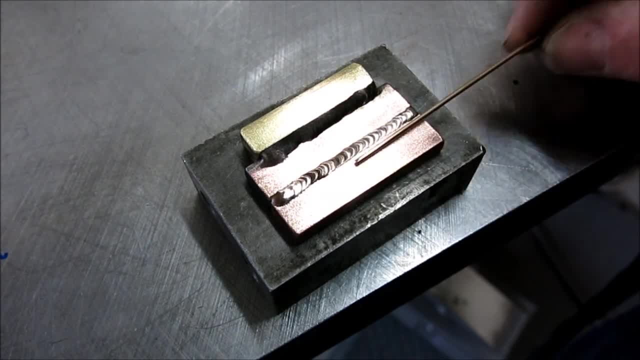 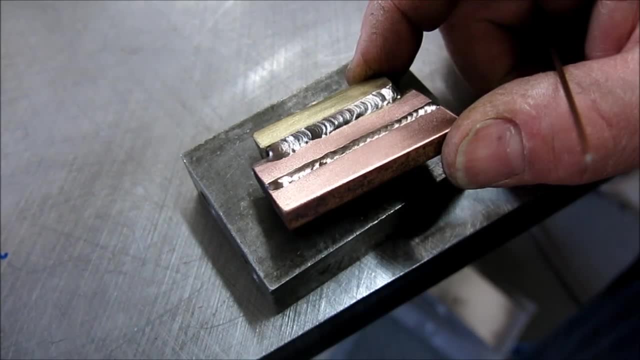 you end up with a dark line where this material is, or a darker line. So that's what I mean by color match. Maybe this doesn't illustrate that well, but anyway, there it is. So now let's go over and let's try breaking some of this stuff and see what we get. 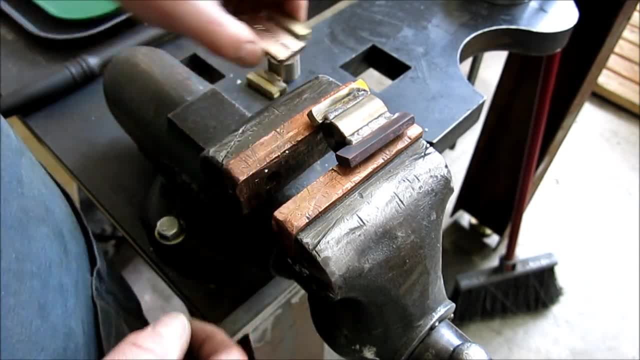 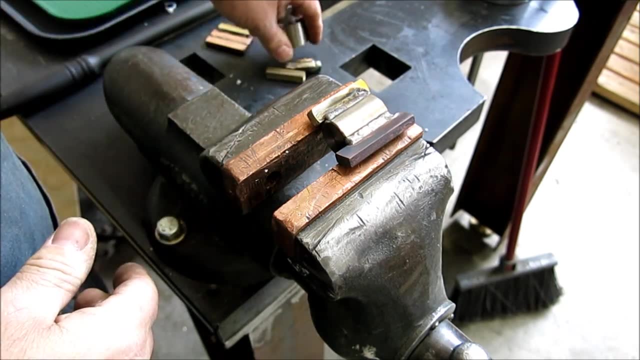 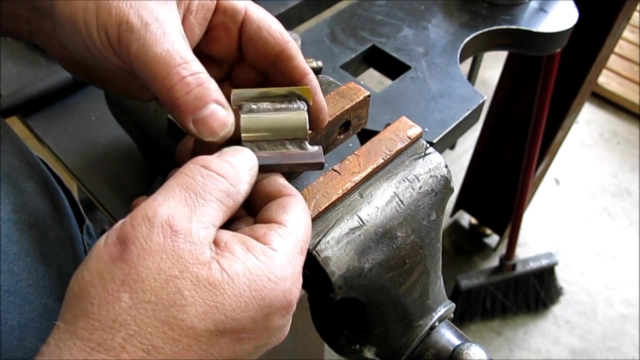 Okay, so here's our samples here. First things first- and we broke this other one- This was the silicon bronze here, So this one here is this: 5% silver, 89% copper, 5% phosphorus. We did the brass to stainless. 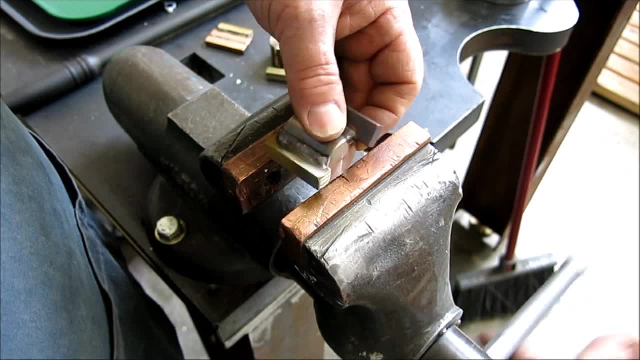 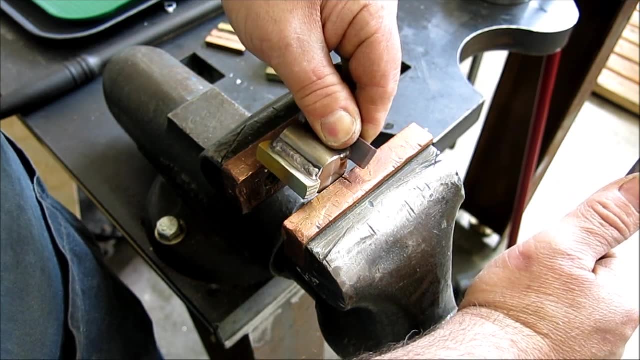 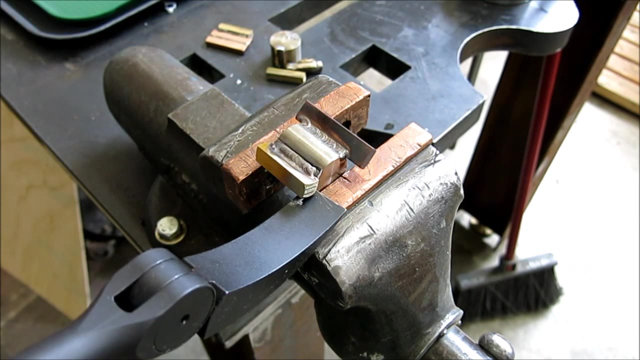 So let's pop that one first and see what we get there. So if I can get underneath there Something like that, Let's try that. Let's see if we can lever that loose. Oh yeah, that one comes loose pretty. 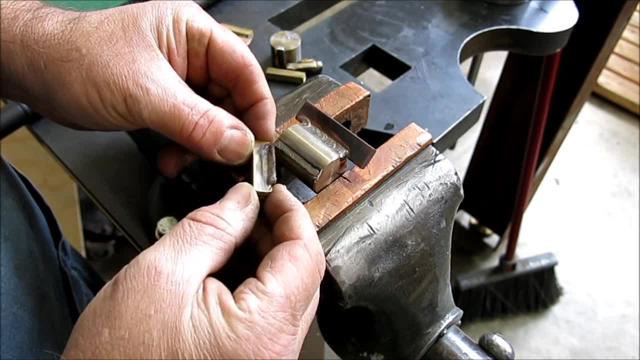 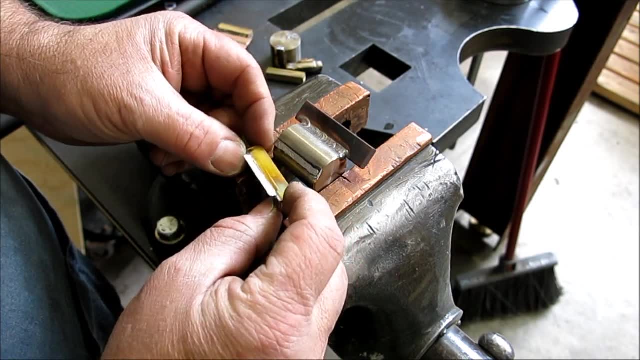 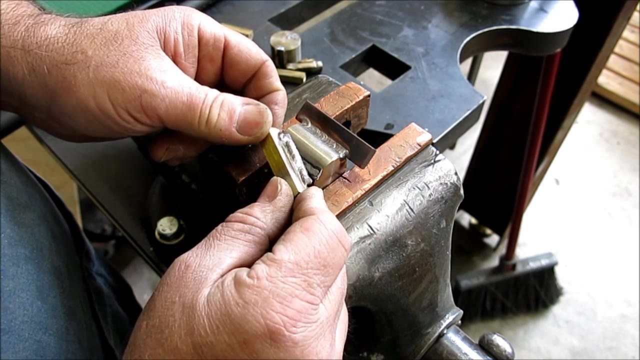 Pretty easily And we get a separation right at the stainless steel interface there. So remember: this is brazing material here. This isn't welding material. We're not welding here. This is a. it looks like a weld, but it's not a weld. 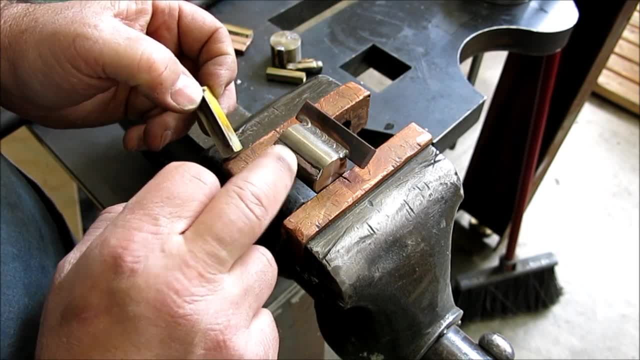 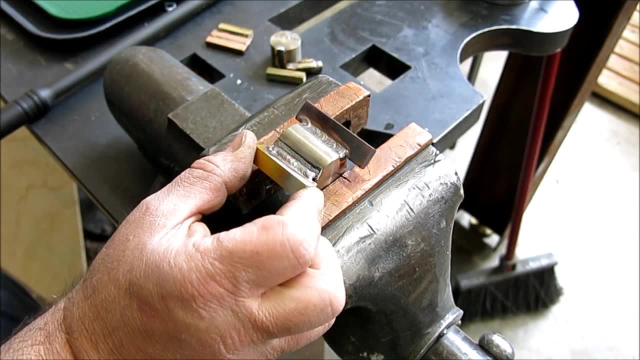 Okay, and there's the inside of that, So it looks like it pulled up a little bit of the stainless- Hard to say. I made this be arcs. It's going there, I don't know. Anyway, it has some strength, but not a lot. 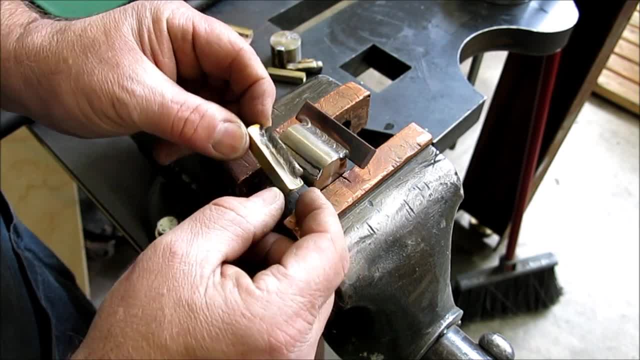 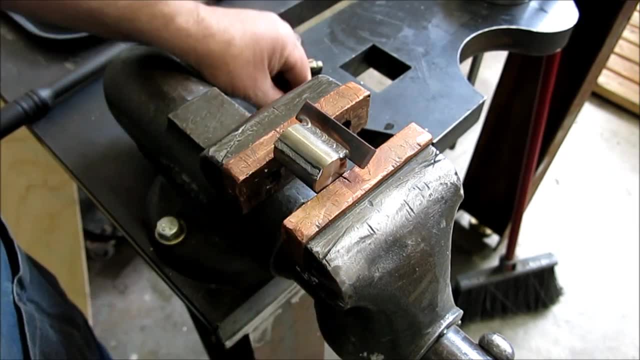 But you know we're torturing that joint pretty, pretty, pretty hard. A weld on the other side would increase the strength dramatically. Let's try the copper now. Actually, you know what? I'm just going to leave it right there. 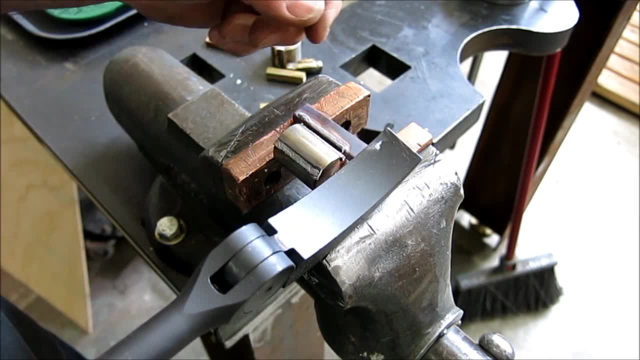 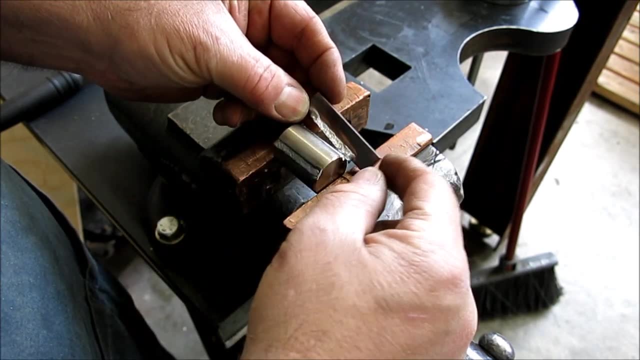 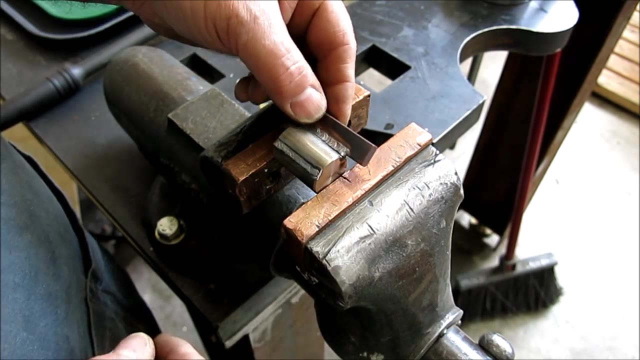 See if we can get underneath it and get this one going. Oh, same thing. So that one The copper, The copper side of the joint is pretty good, but the stainless steel side of the joint is not so good. But once again a very, you know, a serviceable joint for non-structural kinds of applications. 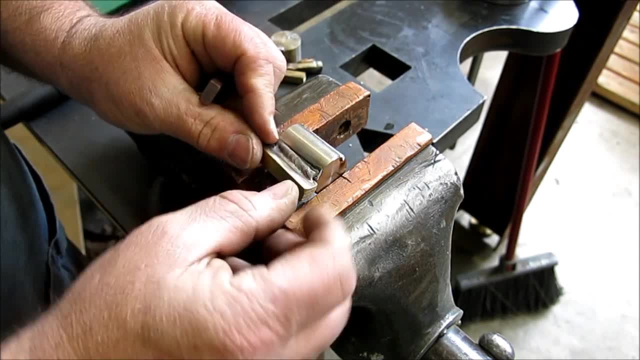 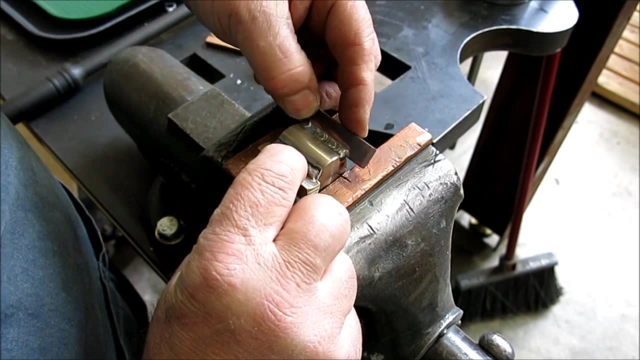 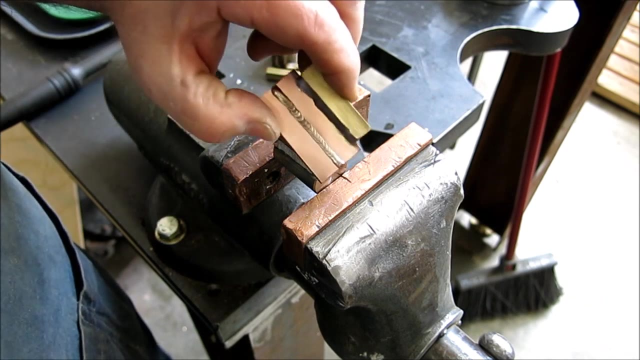 Let's see, Put that right back in there. Yeah, it's a clean fracture. Yeah, Boink. Okay, All right, Let me reset the camera and then we'll try this one here. Okay, So let's pop this loose. 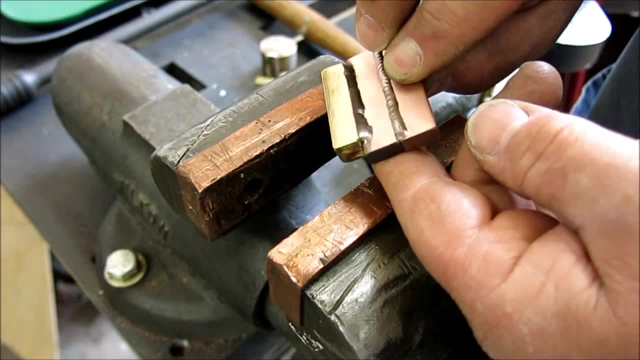 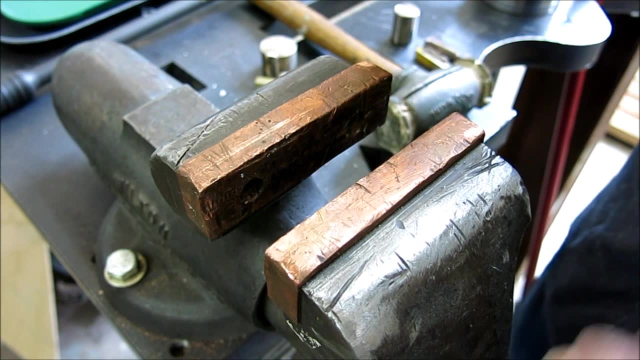 So let's do the brass one first. So what I'm going to do is I'm just going to clamp it like this and then I'm going to knock it over with a hammer. It only took me about a half an hour to pick out which hammer I wanted to use. 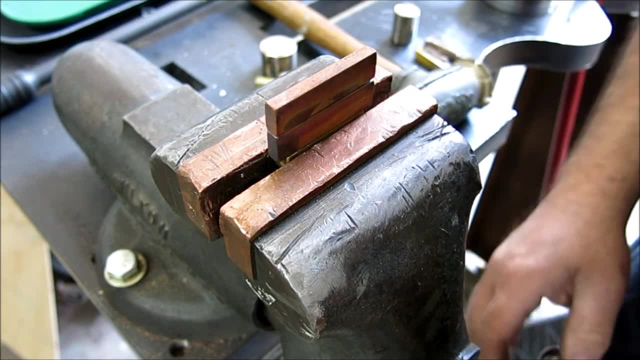 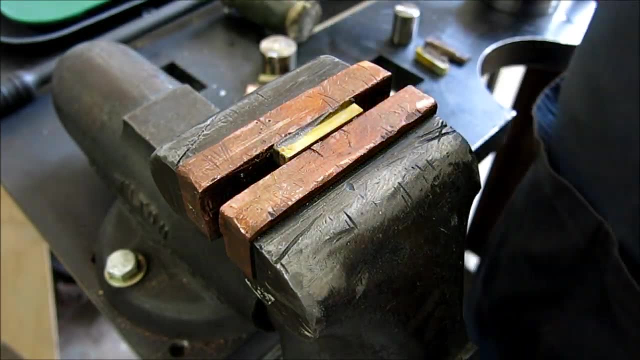 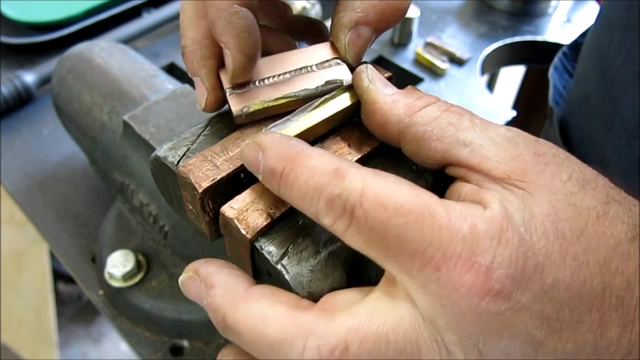 I have so many choices, All right, So that puts that pretty good. So let's just, Let's see what we get. Boink, Okay. Now this one, Let's see, Let's get this back up here. So this one kind of well, it came apart in a different way. 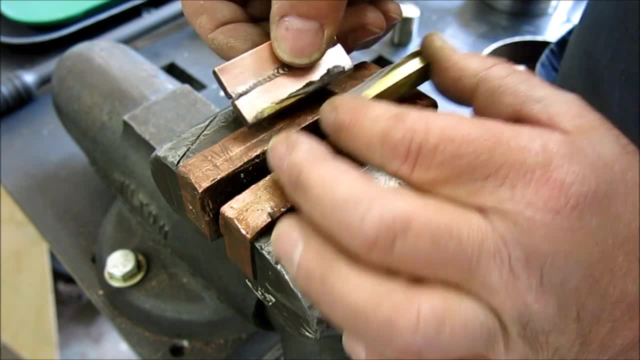 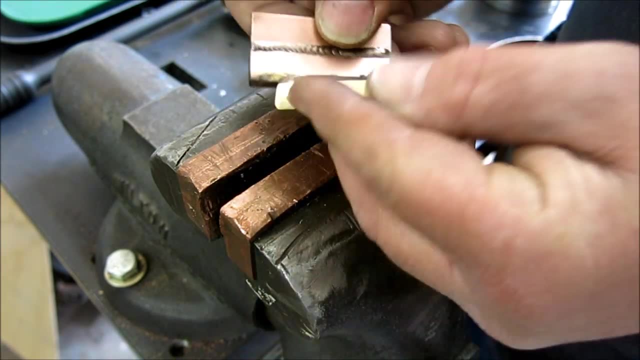 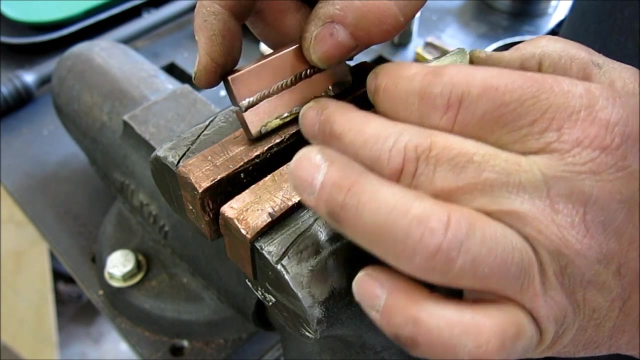 So we came off of the brass and then we got into the copper. So this is probably closer to the ultimate strength of this material. Let's see if we can put that back together there Like that. But it's a brittle fracture through that weld. 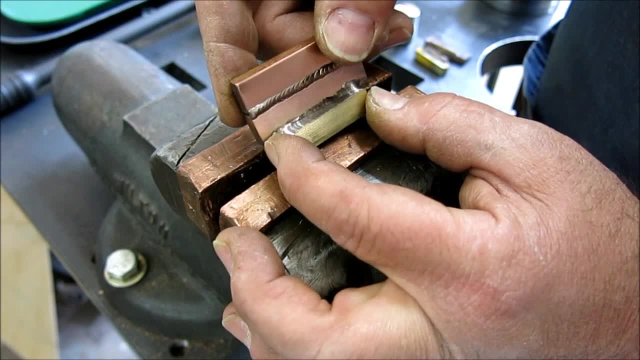 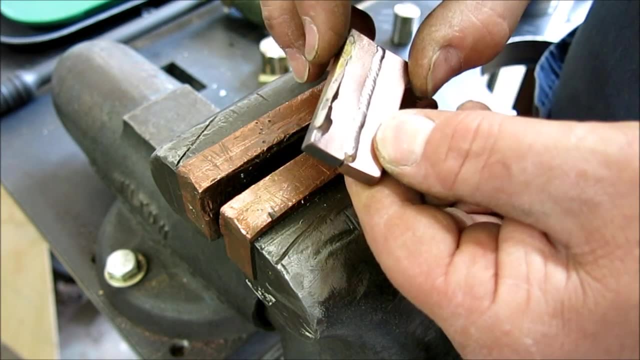 So this material is not real ductile. I can say that, And as I started to hit it, I hit it a little high and we opened up this copper one too, So let's do that one next while we're here. 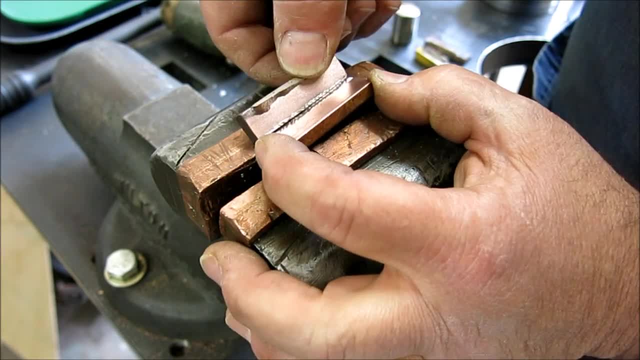 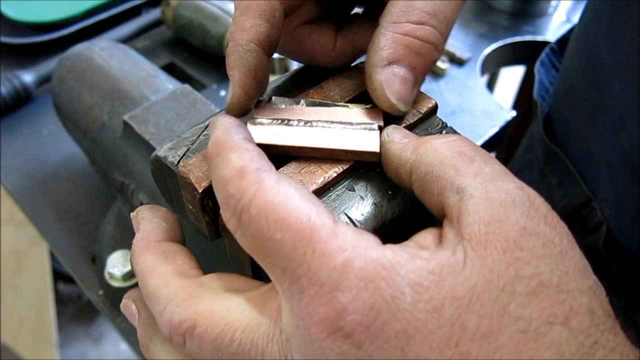 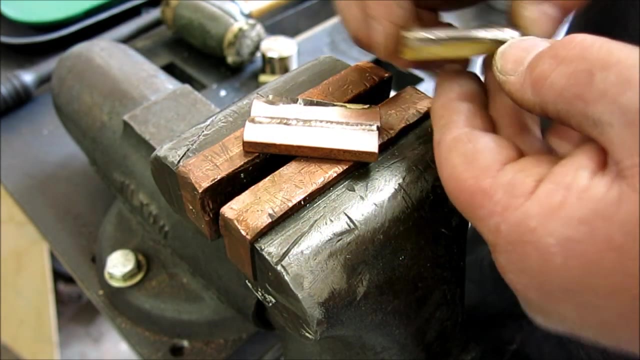 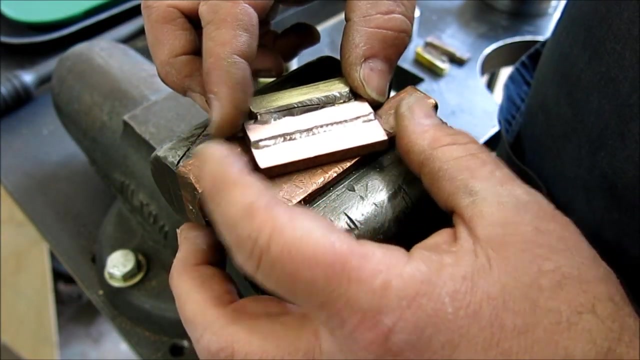 Flip that over. Yeah, Boink. Okay, So the weld lacks ductility, but it does make a joint. If the joint had its own mechanical support- you know a tube inside of a bore or something like that- where it had its own mechanical support. 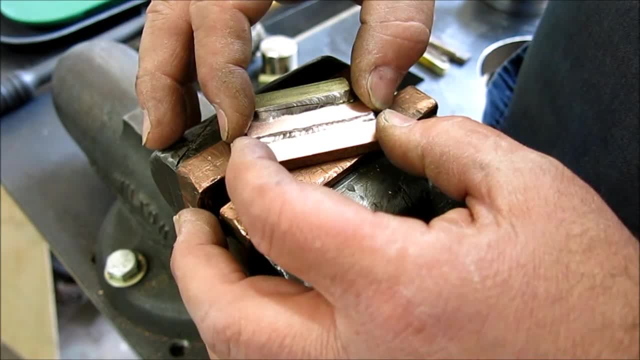 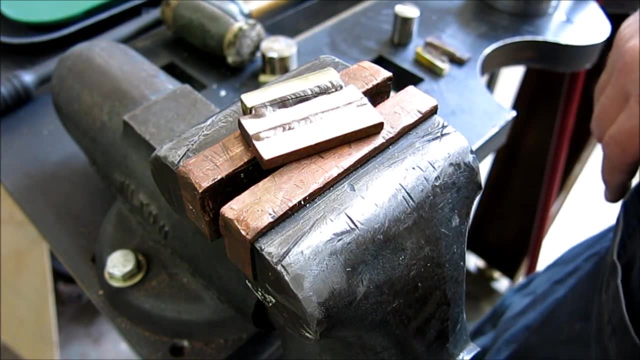 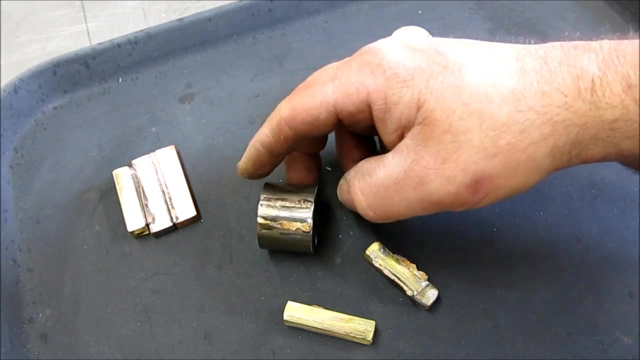 and all this weld was doing was sealing it or joining something it would perform pretty well. Don't weld any lifting equipment with this material here. This is probably not a good choice, Okay, Okay. So here's our test victims here. This was our original silicon bronze stainless steel to brass that we broke apart.